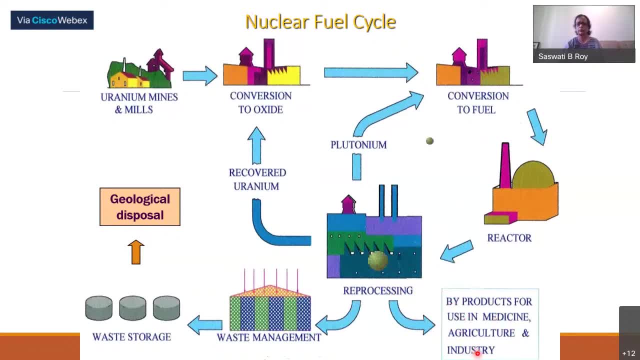 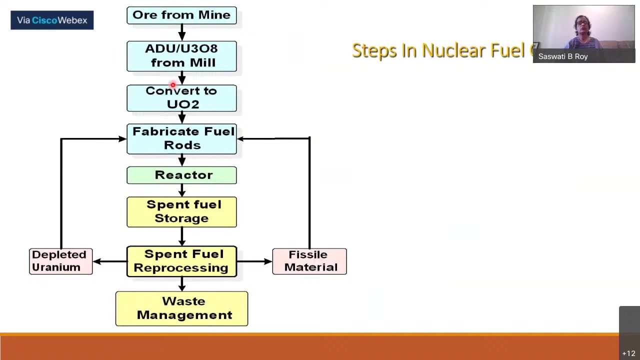 not directly from the power point of view, And there is some storage outlet for the storage of the material which may be of use in future or for the time being as a sourced waste material. So in the fuel cycle we have seen all these steps over some mill conversion fuel dot. 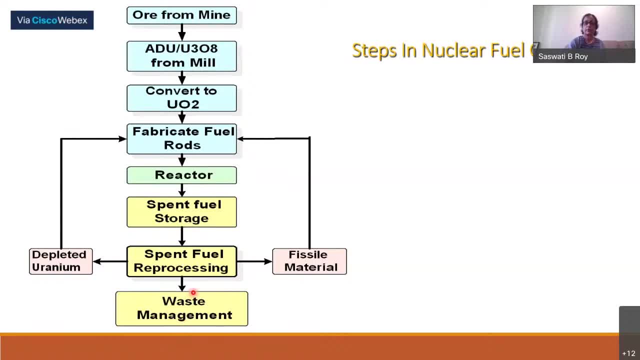 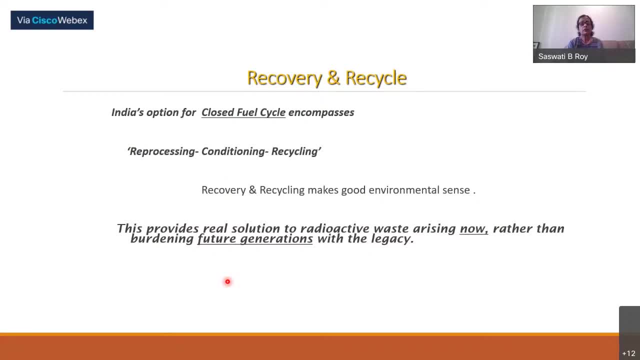 reactors, paint fuel processing, and today we are doing that. So this is our present fuel cycle. We have seen all these steps over some mill conversion in that waste management Here: recovery and recycling. This India's option for closed waste recycling encompasses reprocessing, conditioning recycling, because this provides 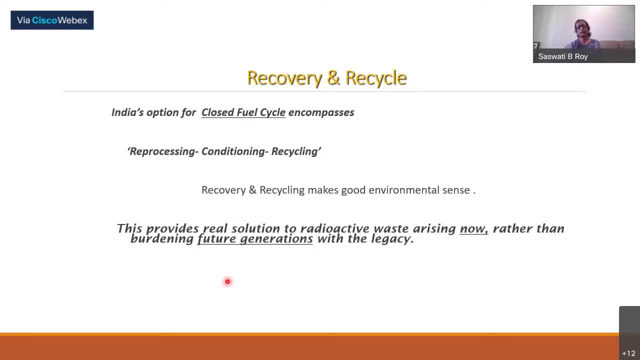 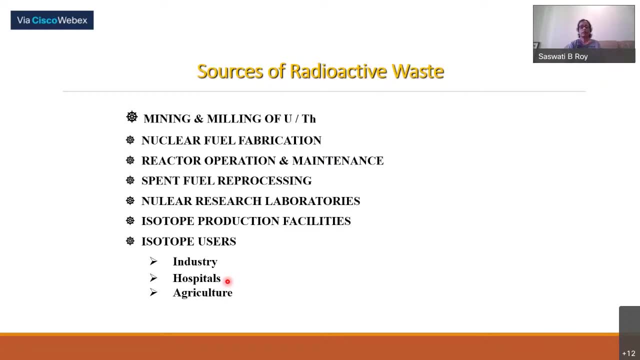 a real solution to radioactive waste arising now rather than burdening future generations with the legacy. The source of radioactive waste in this nuclear waste recycling is every point. we will be generating some amount of waste material, but most importantly is in this area the spent fuel represent. So we will concentrate on that part. Others will. 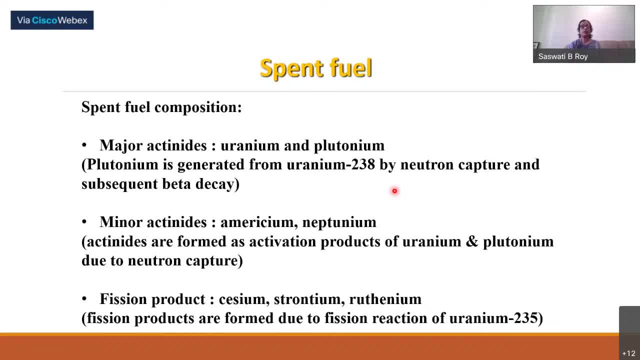 come automatically within this. So spent fuel composition, as we have already learned. this is major actinides, which are uranium, plutonium, which is during reprocessing- we have already recovered, Maybe some small amount there in the waste- and then minor actinides. 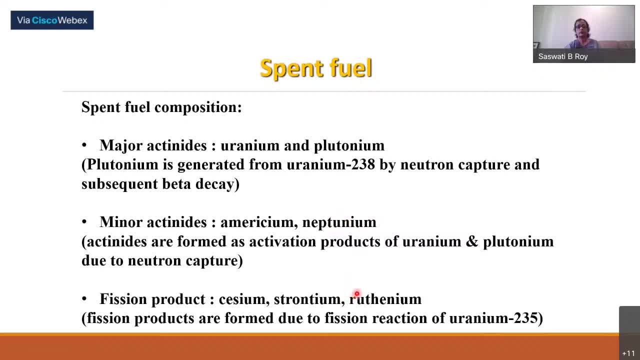 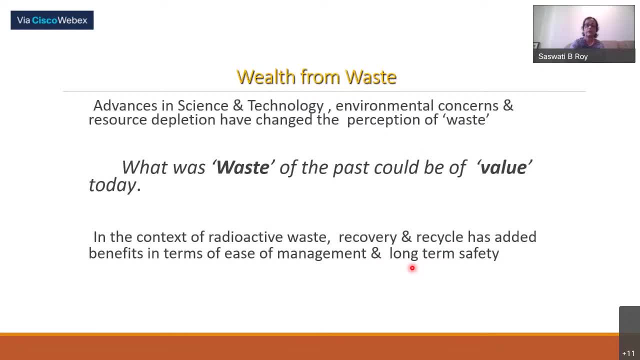 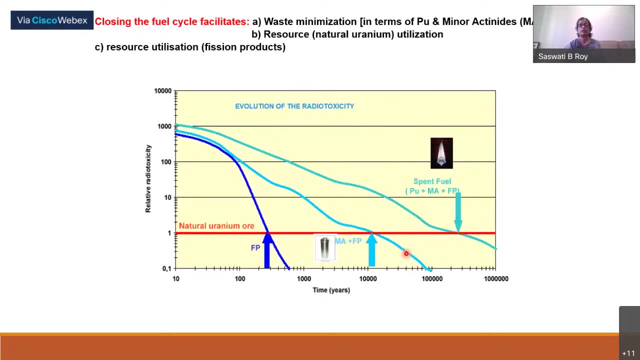 that has gone to the high level waste and patient products that is also there in the high level waste. So, as we said, that what is waste today, but what was waste for the first could be valued today. So we will try to generate that concept Now in this. this. 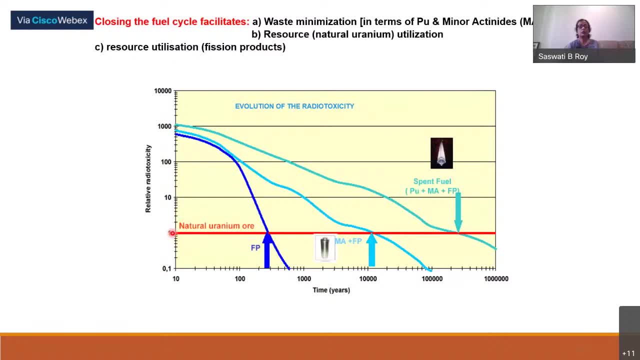 is a diagram where we should have shown you that radio related radio toxicity of natural uranium ore is at this line And if we take our waste fuel with all plutonium and your plutonium, minor actinides and patient products, we can see it will take nearly 200,000 years. 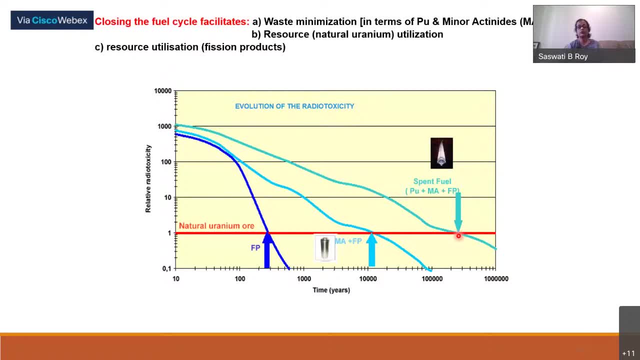 to reach this level, this radio toxicity level of the natural uranium ore, And if it is, plutonium is removed. only fuel is removed. Okay, If it is with minor actinides and patient products, then it is taking 10,000 years. And if we remove, 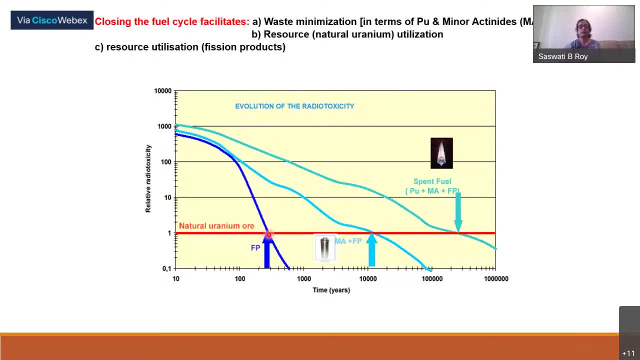 minor actinides also from there. it is only with the patient products. then it is coming within 300 years. So we can save so much of storage space and time If we can remove minor actinides from our waste material and spent fuel material. So one by one we will see that how. 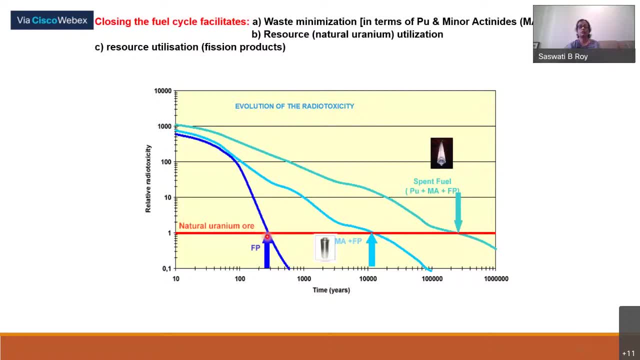 the effect of the waste material will be. We have seen that what can happen to waste material is much more destructive in longer time time period because it is sold, it is destroyed. Then under in the process block diagram we observe the effect of different elements which we take out on our waste fuel. 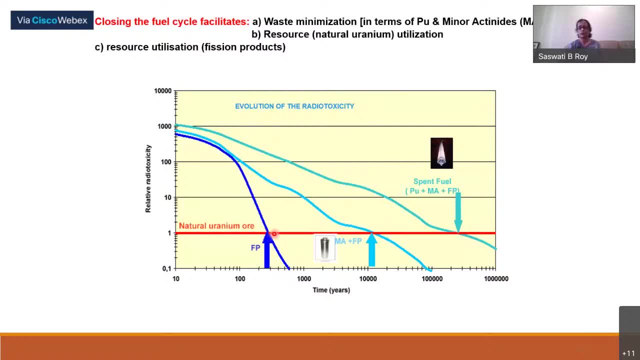 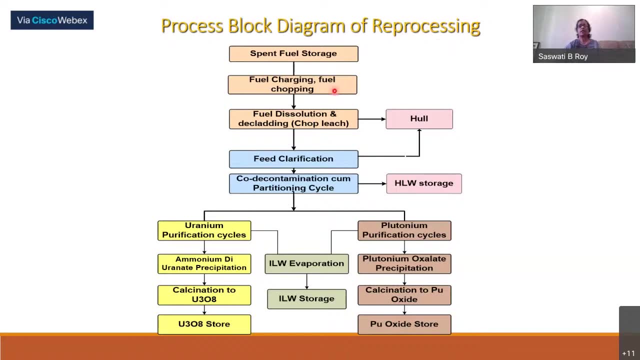 or the spent fuel and how it will help in our management of the waste. So in the process block diagram I will, if you recollect, we have seen that our major ап*** runällt- This was hull, which was from the dissolution that solid material then eat. 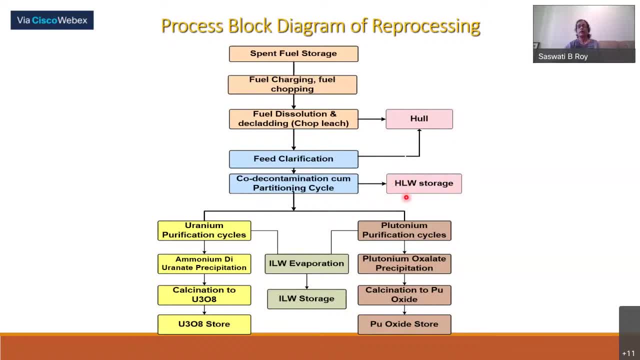 has always been taken. Basically it was big. Compare another example: The700 1D management tool, and we can see that we had all. this provides much more a load. it was high level waste which is generated during the partitioning cycle of our process. 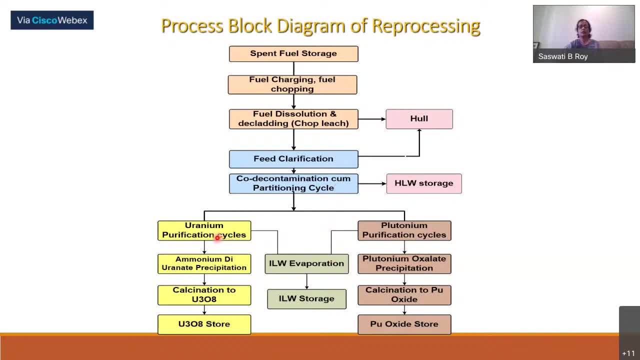 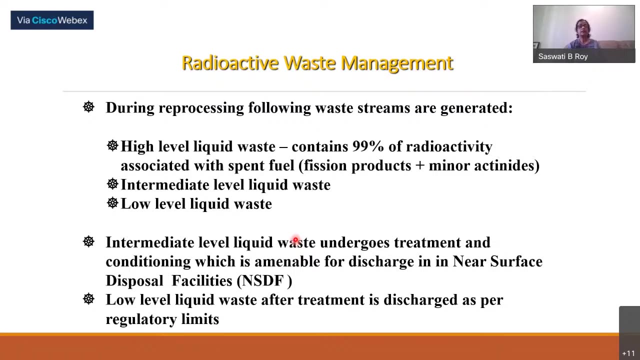 And during the processing of uranium and plutonium to take them in their pure oxide forms, we have generated some amount of intermediate level waste and low level waste. So in this we can see that 99 percent of the radioactivity has gone into the high level. 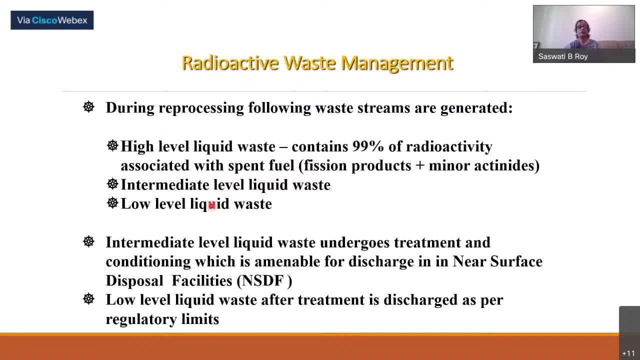 liquid waste, Intermediate level liquid waste and low level liquid waste. they contain very less amount of radioactivity And we have seen that intermediate level waste that can be conditioned at the process with conventional processes like selective precipitation, barium chloride or ferrocyanide, or membrane separations, even concentration by evaporation. 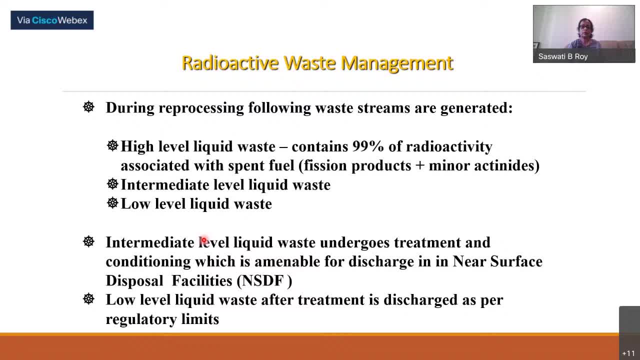 Similarly we can concentrate the radionuclides from this waste and then we can just condition them in matrices like cement matrix and then we can put them near surface disposal facility there of that level And liquid level, low level liquid waste. they don't even need that. This can be primary after. 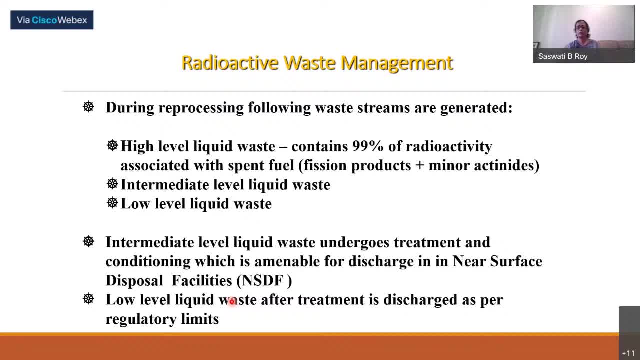 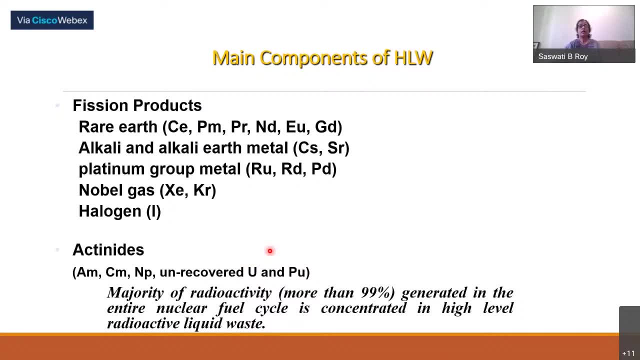 primary treatment dilution. They can be reused or disposed as per the regulatory norms. So major concern is only with the high level waste. The high level waste. they contain rare earths, alkali alkaline art metals, plutonium group metals, noble gas, halogen actinides, In that these are 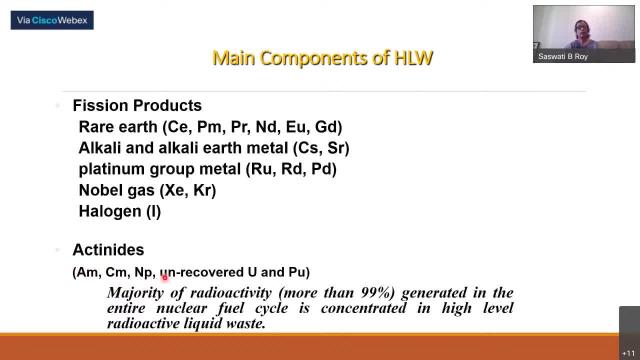 presence in the air and at the center of the material are all cashmere: actinides, Amnesium, LDobemonic, Nioptonium, protein val prime Neutronium and some unrecovered Uranium and Plutenium. That may be very small quantity, but still they are there. 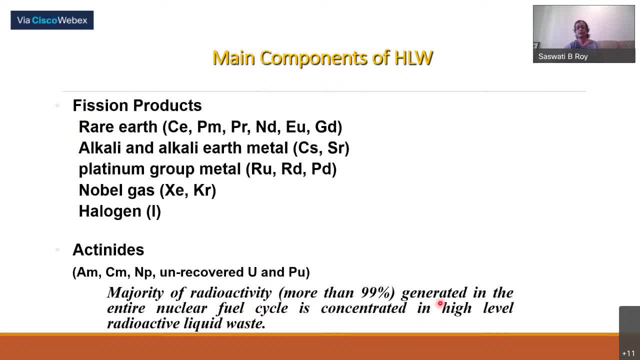 So with this composition our management will start, because majority of the radioactivity- more than 99%- generated in the entire looks at it- is concentrated in high level. So high level radioactive waste management below 70 percent of all these levels would be. radioactive waste is very common here in our country. What we such to do is by adopting 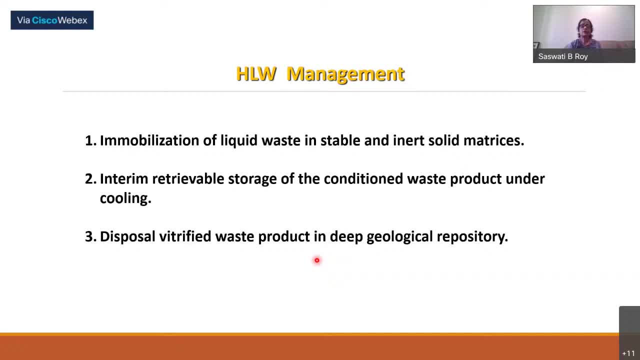 self-енное einzigart���em: purely benign culinaries that contain high level, more or minor dicu dane. as to a type alternative of is problematic to these items are probably the most significant qualities, as in this way: immobilization of the liquid waste in stable and inert solid matrix. Now, 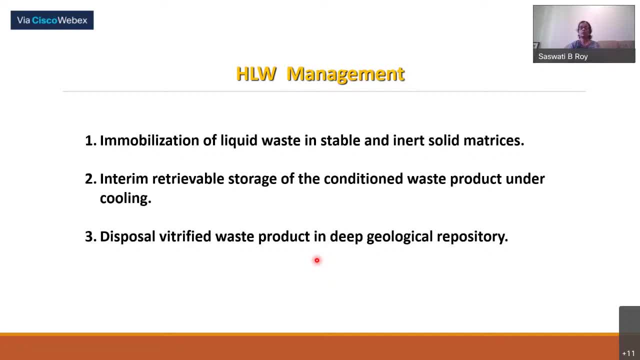 this inert solid matrix has to have some special properties, like they have to be radiologically stable, chemically stable, thermally stable. They should have very good volume reduction factor, They should have a very good waste loading factor and, on the top of everything, 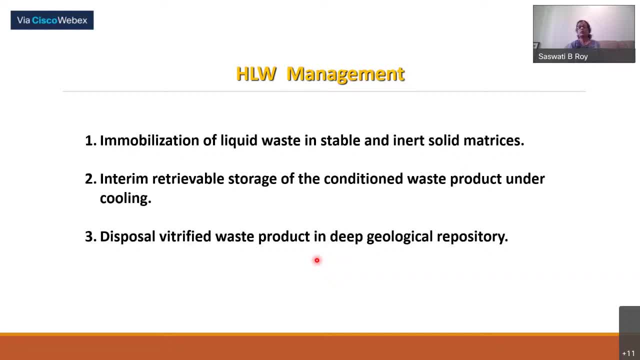 they should be economic also to use it for the prolonged life. So based on all these considerations, as you know, glass has been considered as a suitable matrix and after immobilization of this waste, it will be kept in the interim retrievable storage for cooling, because you know, if you it cannot be cooled, then they may lose there. 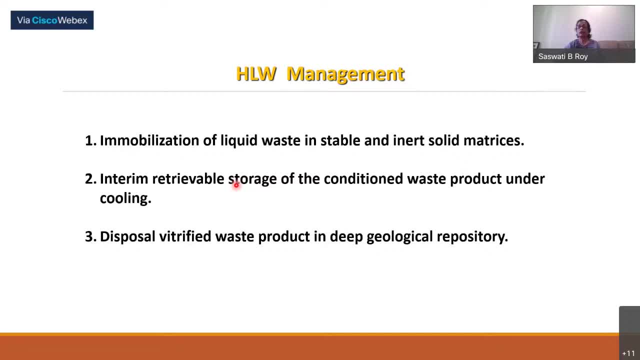 These properties because of this continuous heat generation and central line temperature will increase. they may lose their chemical stability. So it has to be cooled and for cooling the special interim arrangements with air flows are maintained so that they can come down to the required level. and once they come down to that required level then it can. 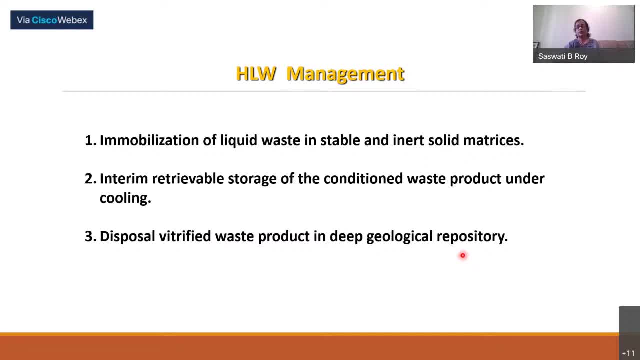 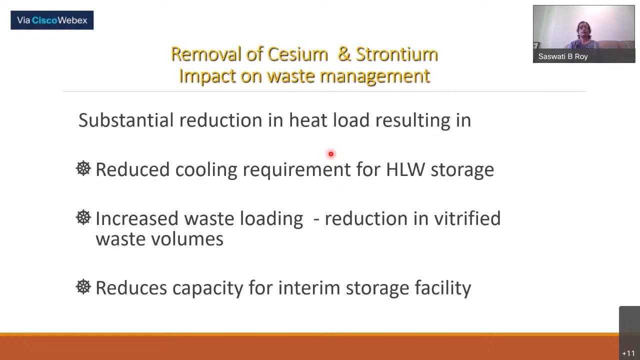 be disposed to the geological repository. So during this processing we are again seeing that what all we can restore? So part of the energy generation processes. now what you can do is you can use these products So you can see the, the, The, The, the. 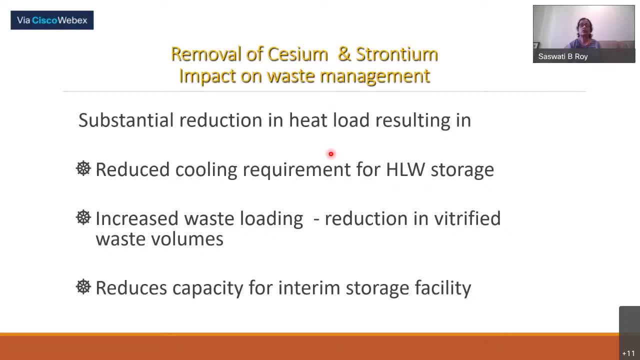 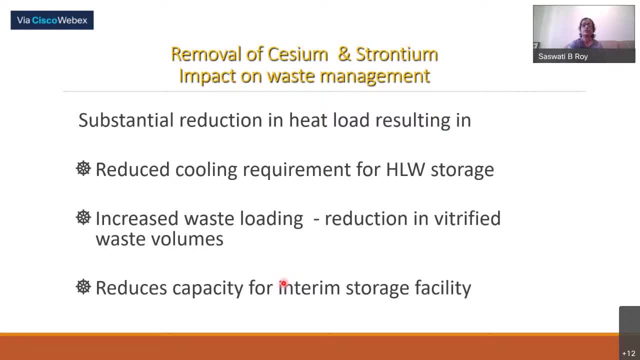 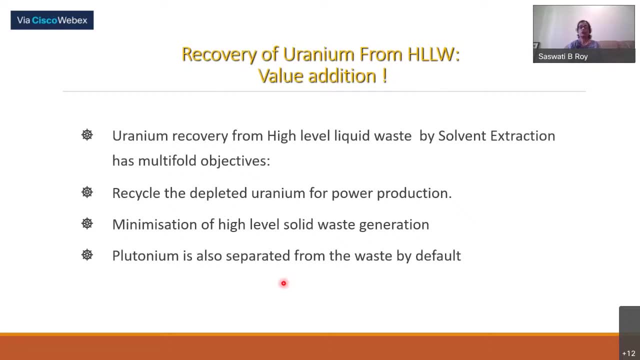 So the first point: we will see that cesium strontium removal, And before that we have uranium plutonium also, which also if we can remove, then it will recycle the depleted uranium and power for the power production. 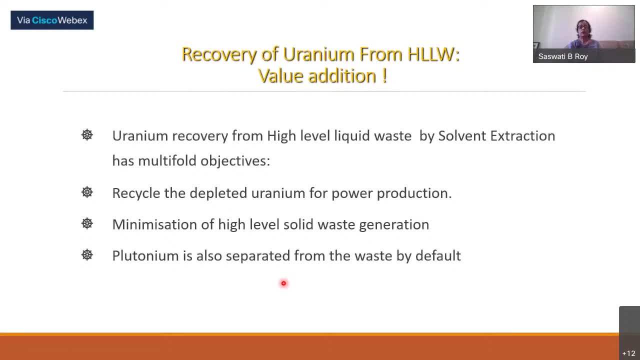 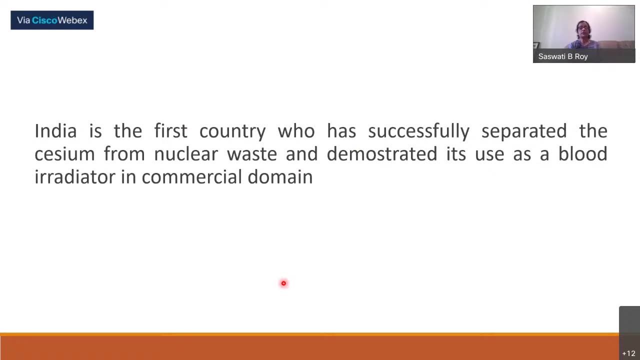 Also, plutonium will be recycled and it will minimize the solid waste generation from the after conditioning of your high-level waste. So, in this line, India is the first country to have a high-level waste generation. India is the first country who has successfully separated cesium from the nuclear waste and 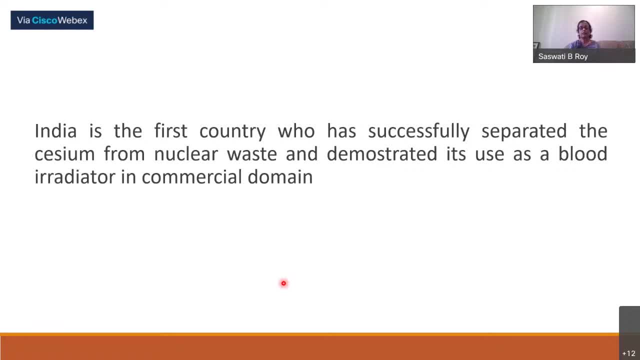 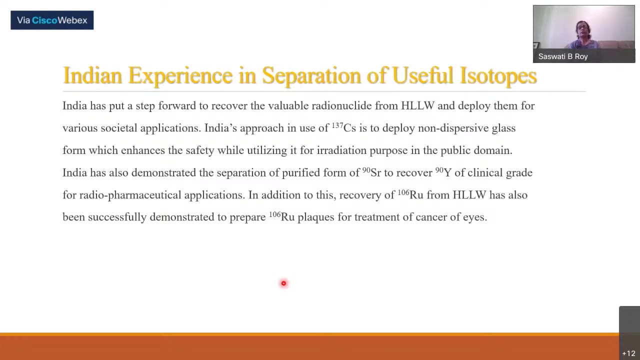 demonstrated the use at the blood irradiator in commercial domain. So, as we said that cesium and strontium removal will reduce a lot of heat load. So this was one of the issues which we started. first, The Indian experience. in the separation of useful isotopes, India has put a step forward. 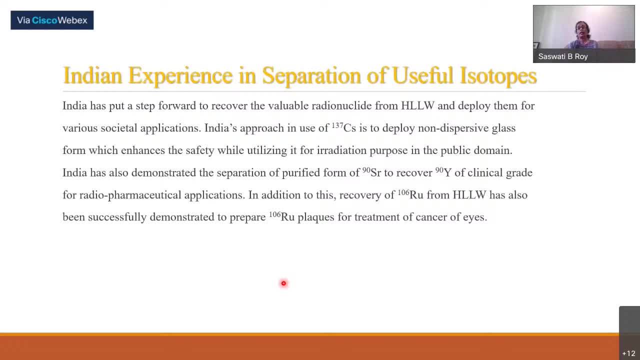 to recover the valuable radionuclides from high-level liquid waste And that is being used for different societal applications. The first is cesium-137, and the second radionuclide is strontium and yttrium, and third is plutonium. 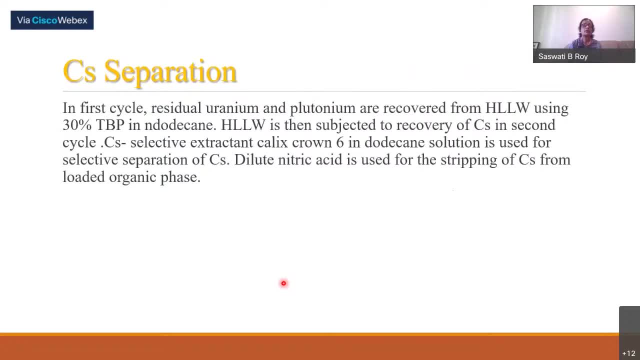 So in cesium separation first, what we do in that high-level waste. it is treated with 30% tributyl phosphate in normal dodecan And treated to remove the high-level waste, The leftover residual uranium-plutonium from the high-level waste first. 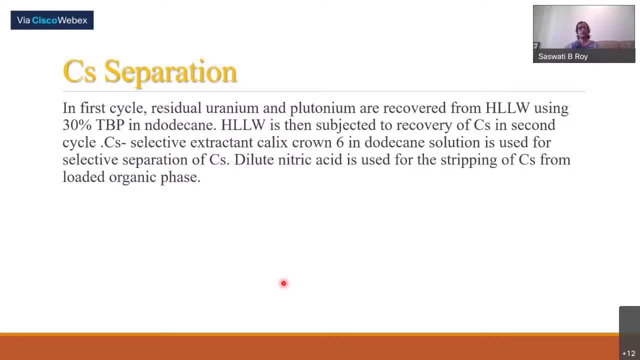 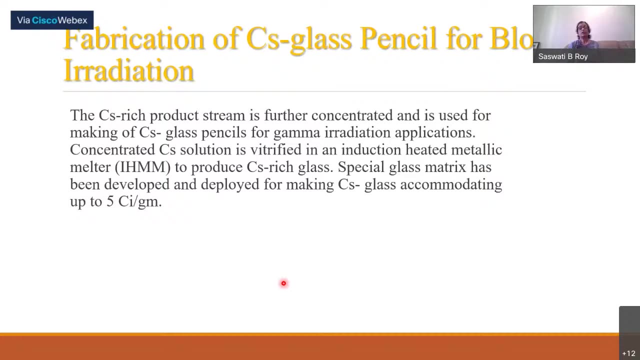 And then it has been treated with cesium-selective extractant. calyx crown in dodecan, solution for selective separation of cesium Dilute nitric acid is used for stripping of cesium from the loaded organic waste. This cesium-rich product is further concentrated and it is used in making cesium glass pencils. 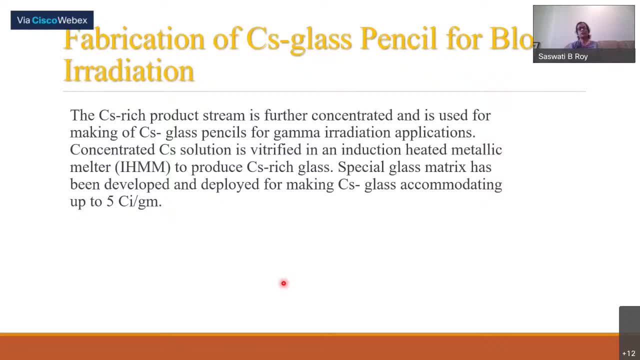 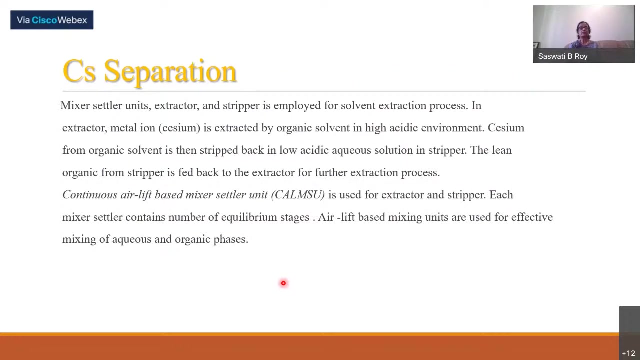 for gamma irradiation Consistency. cesium solution is vitrified in an induction-heated metallic melter to produce cesium-rich glass. Special glass matrix- it is borosilicate glass- has been developed and deployed for making this, And you must have seen it in your earlier classes. that how that pencil is being used. 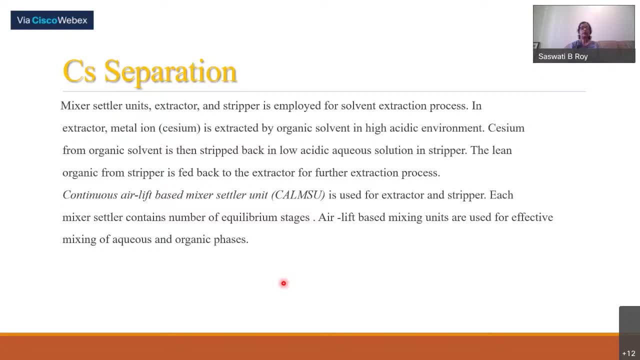 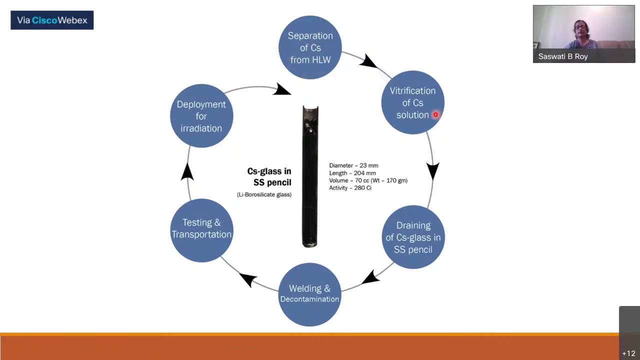 And equipment used here again mixes atlas, The stripping and extractor. Both are mixes atlas with airlift mixes, mixing arraignments, And this is that process: separation of cesium from the high-level waste. Then vitrification of the cesium solution, blending the cesium glass in stainless steel pencil. 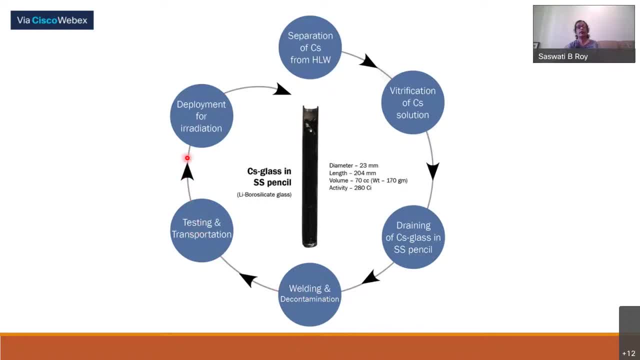 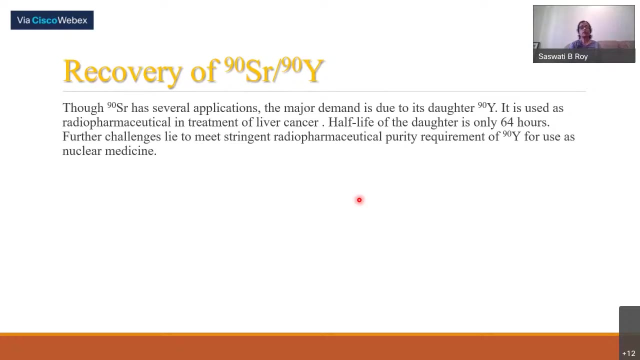 welding, decontamination, testing, transportation and deployment for irradiation. So this is a borosilicate glass with activity around pH security, So this is already been deployed. And the second one is strontium-etrium. Strontium is having its several applications, but major demand is for etrium. 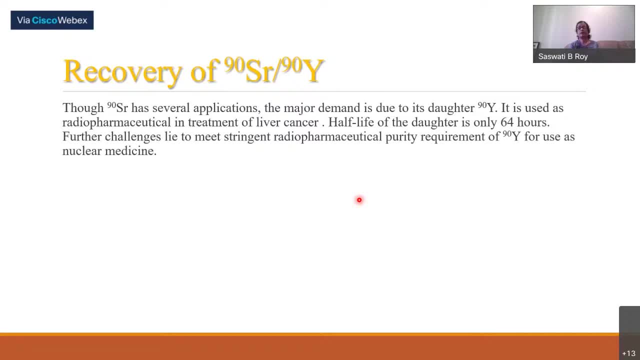 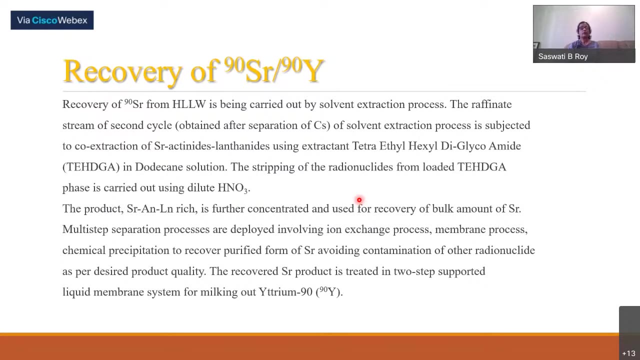 Etrium is the daughter product of strontium, which is having a half-life of a very small a few hours. So part of the challenge is how to make it nuclear pure for radiopharmaceutical use. So this recovery of the cesium from high-level waste. 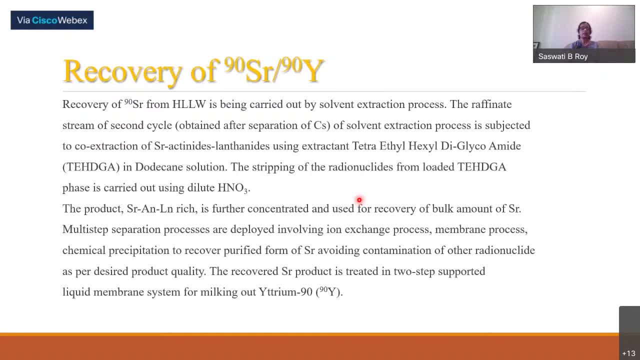 It is being carried out by solvent extraction process, again the raffinate stream of the second cycle. after obtaining the after removal of the cesium of the solvent extraction process, It is used for co-extraction of cerium actinides and lanthanides using TEDDA. 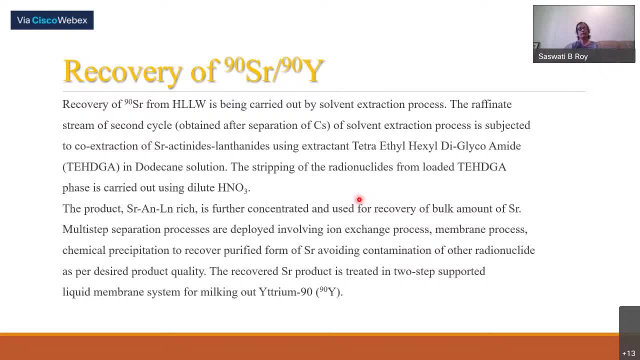 The stripping of the radionuclides from the loaded solvent is being done with nitric acid, And the product- cerium actinides, minor actinides and lanthanides, which is part of the solution, is further concentrated and used for recovery of the bulk amount of strontium. 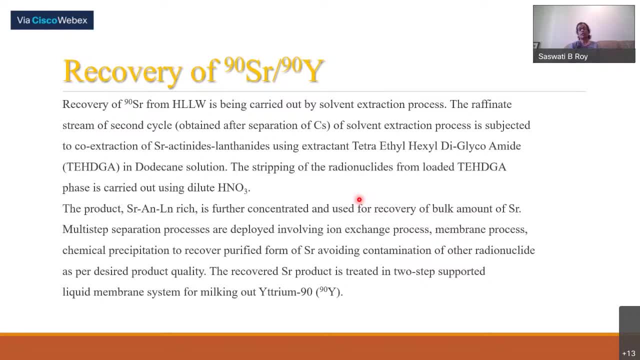 The multi-step separation process are deployed, involving ion exchange process, membrane process, chemical precipitation to recover purified strontium, avoiding contamination of other radionuclides. as for desired product quality, The recovered strontium is then treated in two-step supported liquid membrane systems. 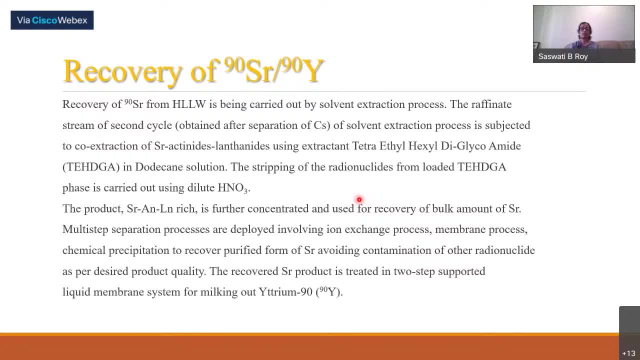 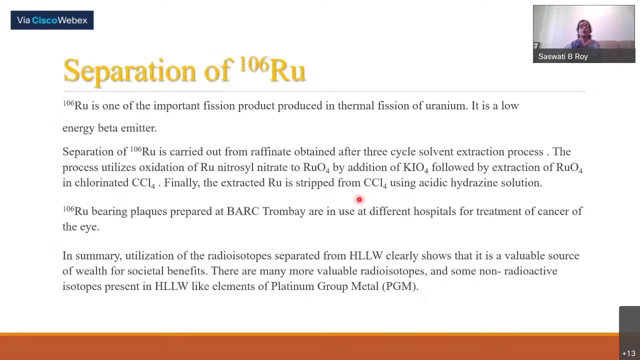 Supported liquid membranes are supported by liquid membranes. Supported liquid membranes are supported by liquid membranes. Supported liquid membranes are supported by liquid membranes. Supported liquid membranes are supported with specific solvent for milking out the atrium of specific grade. The other one which we have separated out is ruthenium. 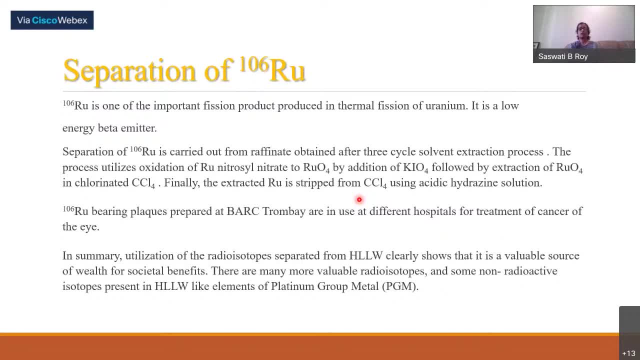 So this ruthenium is also a very important product in the thermal efficient And the separation is carried out from raffinate after three cycles of this solvent extraction And it is first oxidized through ruthenium. Now the first check is to see if the surface area is treated. 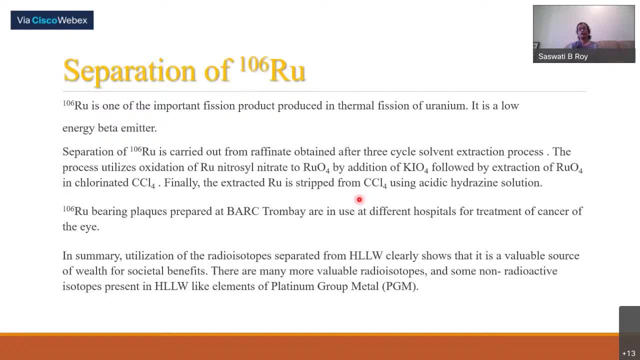 There are very few traces of ruthenium, and we can see that there is a very high percentage of this noise. So what we want to do is to put in a single solution with the support of the various raging, and that is what we have found. 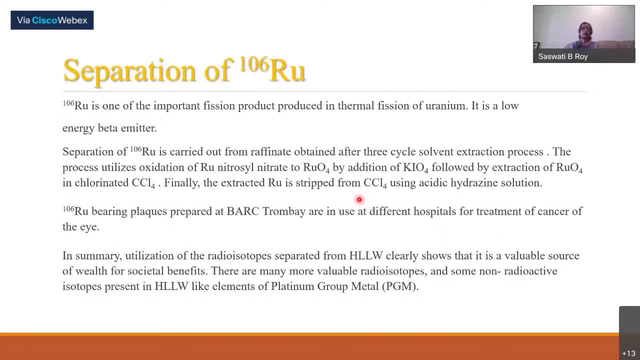 There is a very high percentage or medium concentration of the ruthenium oxide, the valency-8, by adding KIO4, followed by extraction of ruthenium oxide in chlorinated carbon tetrachloride. Finally, they extracted ruthenium and stripped from carbon tetrachloride using acidic hydrogen. 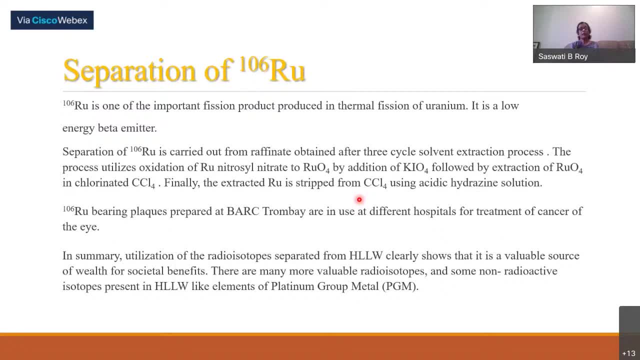 solution. So this ruthenium bearing flick- already we are see Trombay has produced and used it for cancer of eye. So, in summary, utilization of radioisoteric stream isotopes separated from high-level liquid waste clearly show that it is valuable source. 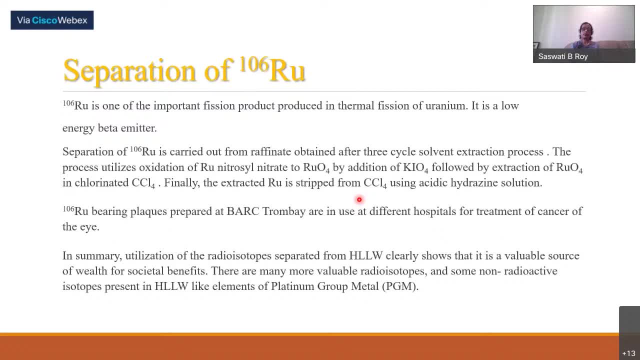 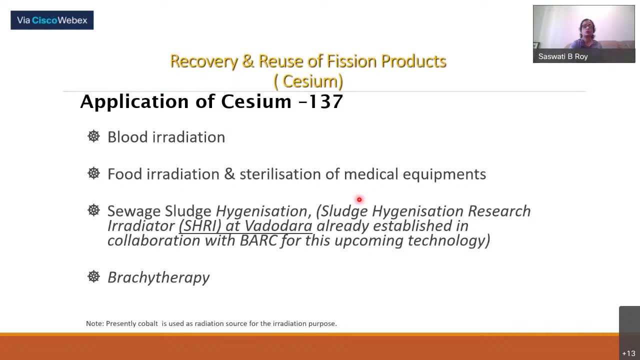 of wealth for societal benefits. There are many more valuable radioisotopes. We can just…. You must have seen also earlier classes. We will go through very fast all this Cysteium we have already seen for blood irradiation. It can be used for food irradiation, sterilization. 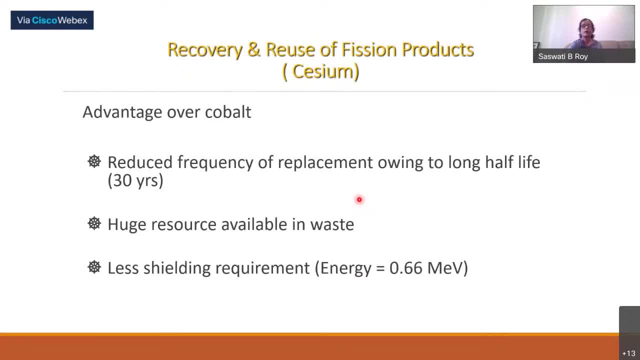 of medical equipment. blood degeneration package therapy. It is advantage over cobalt is this: reduced frequency of replacement to increase longer half-life use, resource available in the waste and less shielding requirement due to energy Strontium also, as you see that 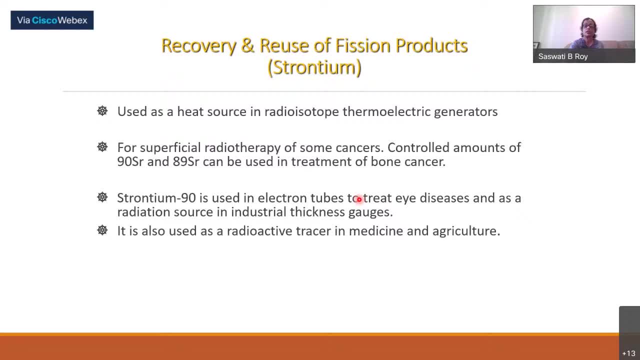 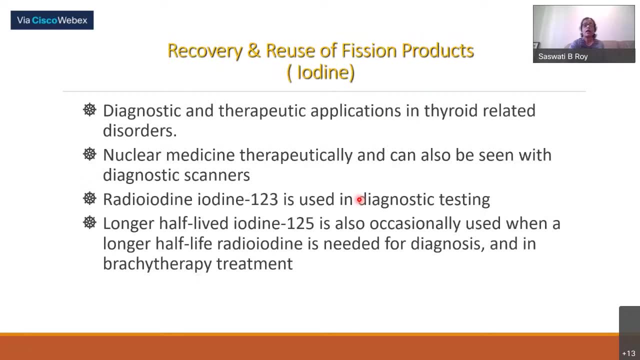 we have so many uses As a radioactive stressor- you have seen in your class- and from there yttrium. This is for this liver cancer, Iodine which has come…which comes from the…their gaseous product or the…from the gaseous product. So this is also very useful for different. 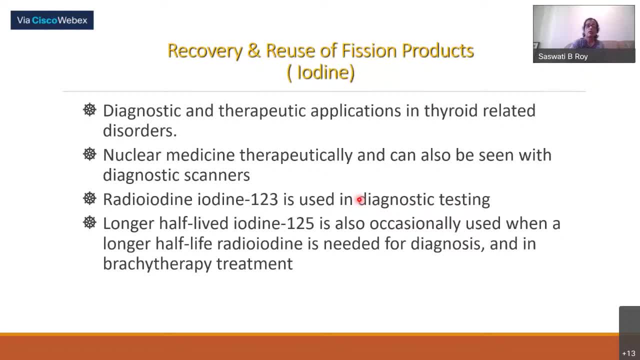 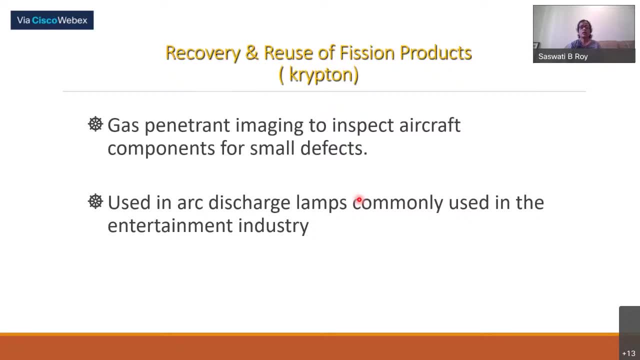 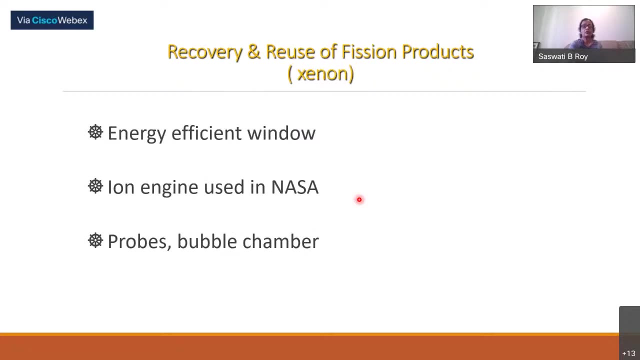 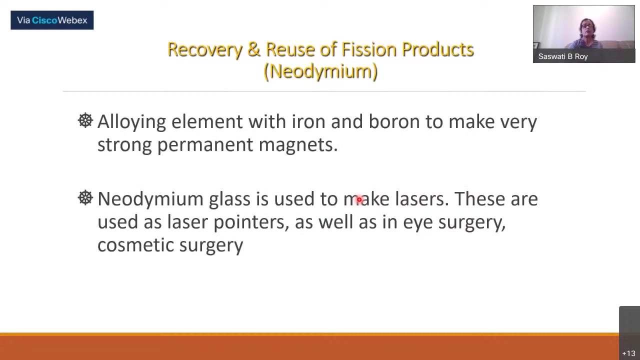 diagnostic applications. Krypton is also coming from the gaseous product. They are used in arc-gestured lamp commonly used in the entertainment industry. Xenon, similarly, can be used from…for many uses, Neodymium is a very important element. 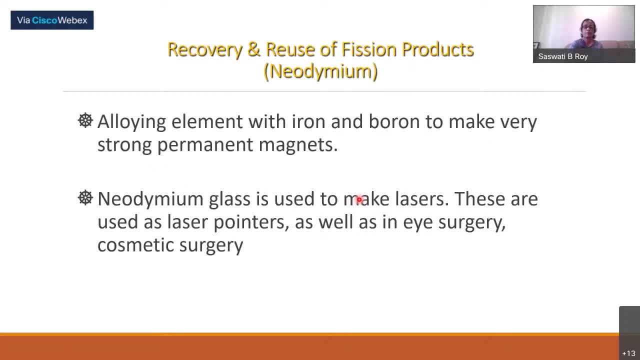 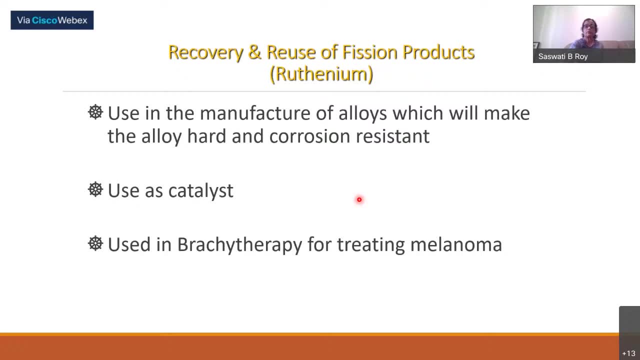 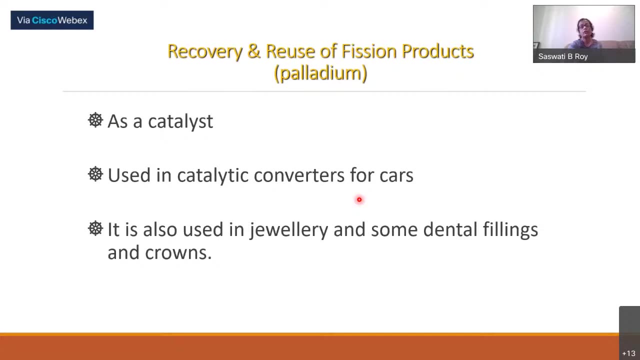 at this moment We are trying for the permanent magnets And ruthenium as a catalyst package therapy manufacture of alloys. Palladium, also catalyst used in catalytic converters of cars, also used in jewelry. Rhodium is also used in catalytic converters of cars, also used in jewelry. Rhodium is 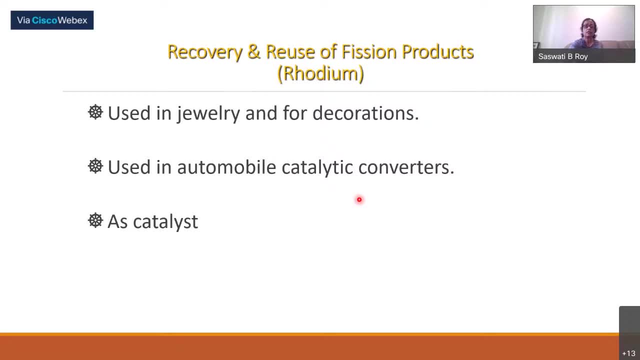 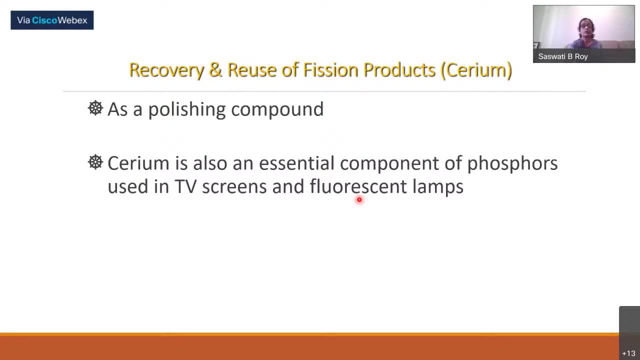 also used in catalytic converters of cars. also used in jewelry. Rhodium is also used in jakbymobile catalytic converters as catalyst Hurdium. as you know, it is essential item for the…the… has a polishing compound also. it can be used. 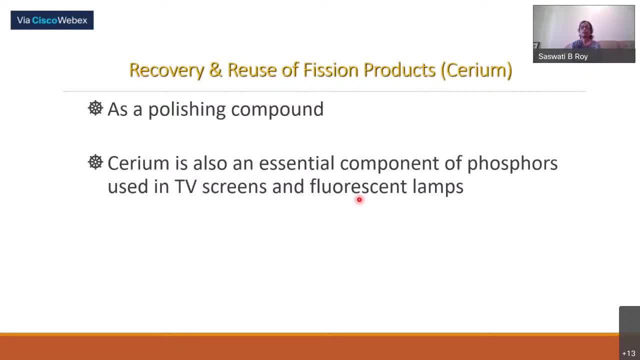 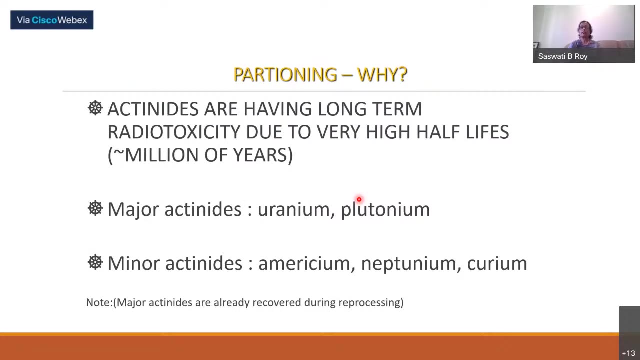 Now. so all these uses we have seen. So once it is taken out separately, we can see that once the separation processes are properly commercialized, it can be utilized in all the steps. P and e夏 don't have to remain as a waste. now we were saying that if we partition this minor actinides, 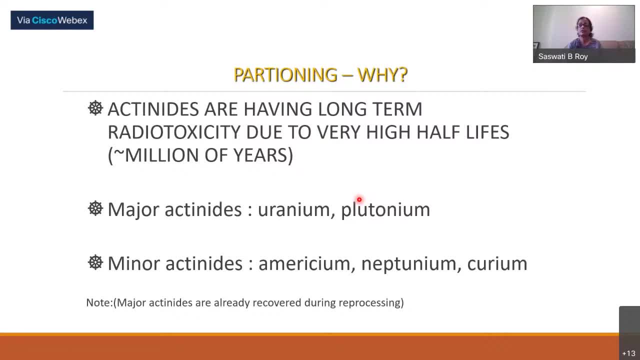 which is there in that high level waste. high level waste as we remember that there was some residual uranium, plutonium, minor actinides and fission products. so, uh, part of the fission products which are high, uh, my heat source generator, like strontium and cesium, can be. 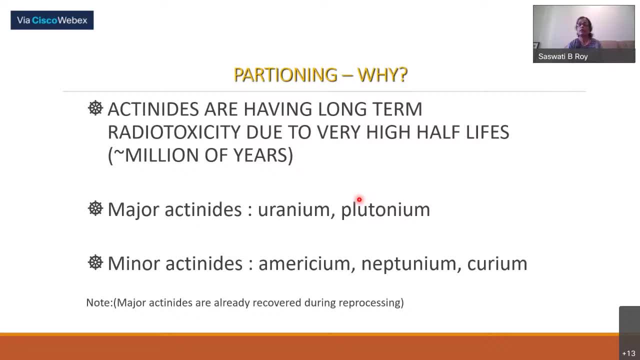 separated, as we have seen, and if they are taken out then their storage requirement will be reduced. and if the minor actinides as a whole is separated, then their storage time is being reduced drastically. you have seen so in this minor actinides, who all are present in 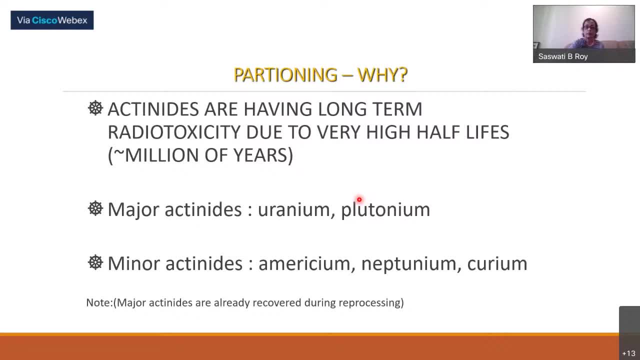 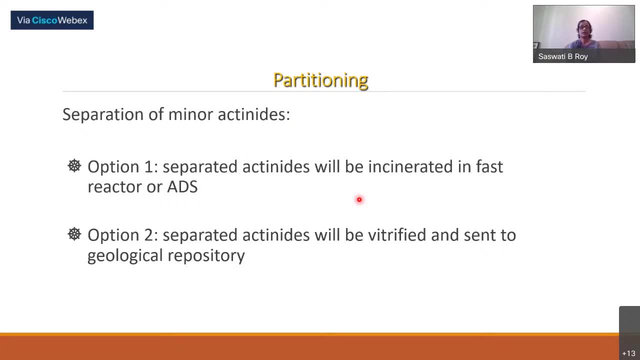 So once they are separated they can be either used in first reactors or radiuses or if they are not used, then at least in a smaller form they can be vitrified and sent to geological repository. But their storage in that intermediate where the heat generation, heat removal is needed. 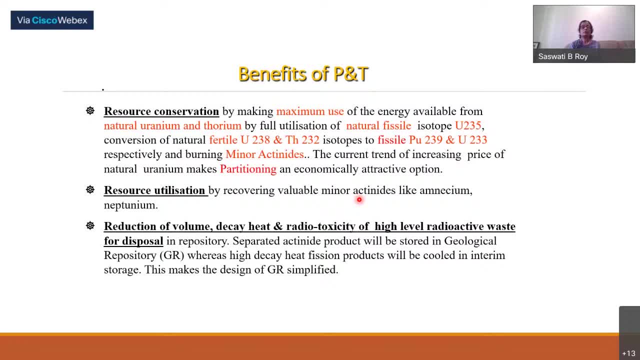 will be much longer. The benefits of the partitioning this is resource conservation by making the maximum use of the energy available from natural uranium and thorium, by full utilization of the natural fissile isotopes And then conversion of this to manmade isotopes- plutonium 239 to 33, and additionally burning. 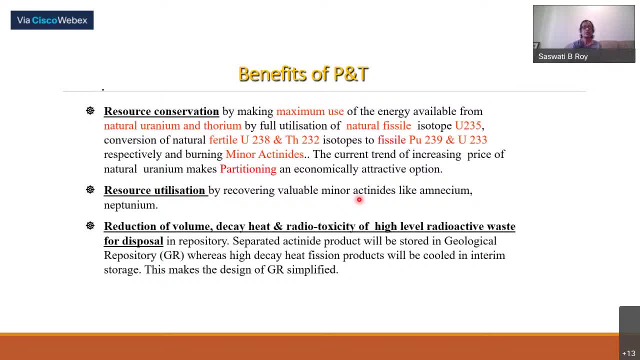 of minor actinides. The current trend of increasing price Natural uranium makes this partitioning an economically attractive option. Resource utilization by recovering valuable minor actinides like ambrosium and mectunium. as we have the users, we can utilize them. 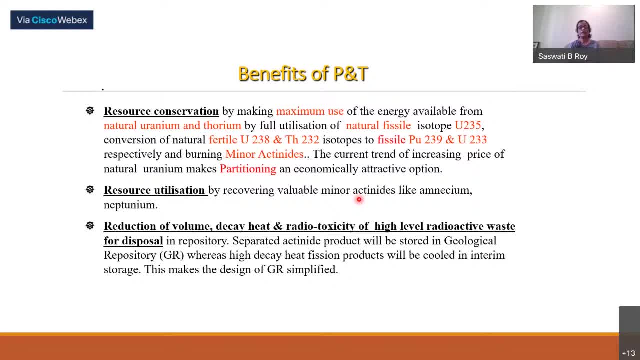 And in waste management. the best use is the reduction of the volume, decay heat and radiotoxicity of high-level radioactive waste for disposal in repository. Separated actinide product will be stored in geological repository. High decay heat fission products will be cooled in interim storage. 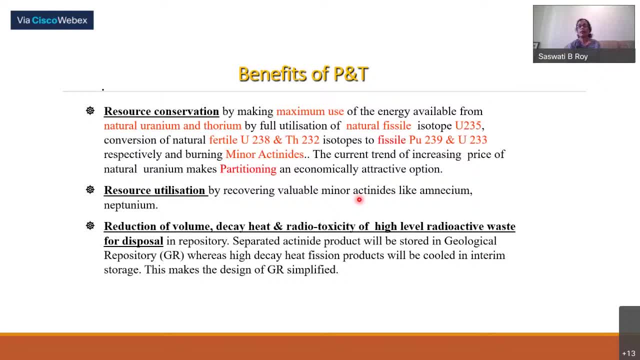 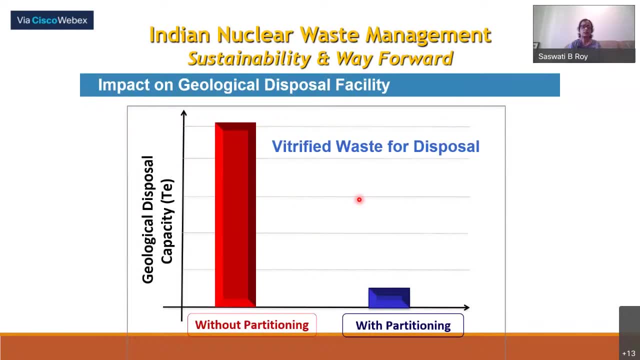 That makes the design of GR much simplified, where that heat removal conditions will not be needed. So if you consider this geological disposal capacity without partitioning, if the capacity would have been this, after partitioning required capacity will drastically reduce. So there is a big use of separation. 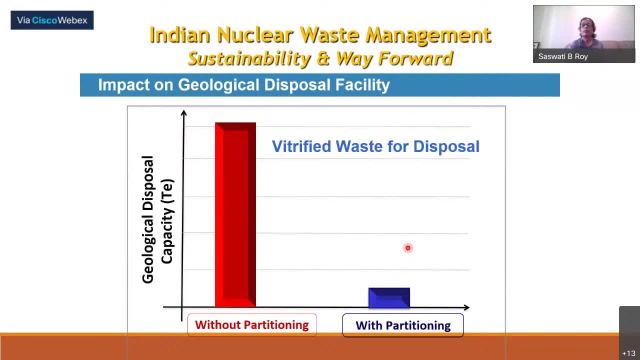 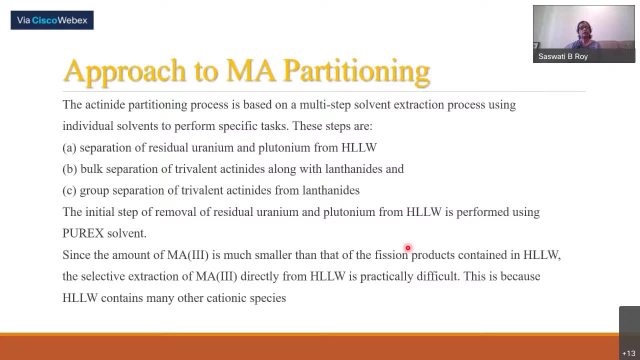 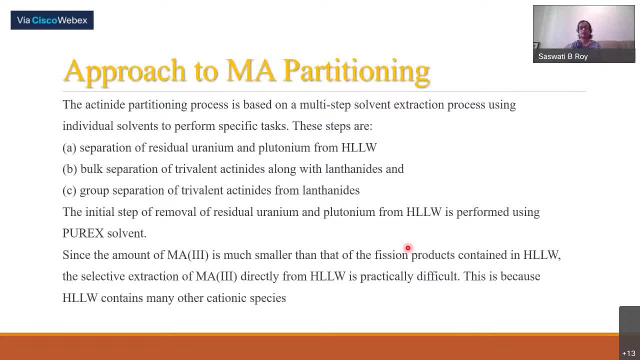 residual uranium and plutonium from high-level liquid waste. this is the first step for all. Then bulk separation of trivalent actinides along with lanthanides. Both are trivalent actually It is difficult to separate, So they'll be separated together as a bulk. 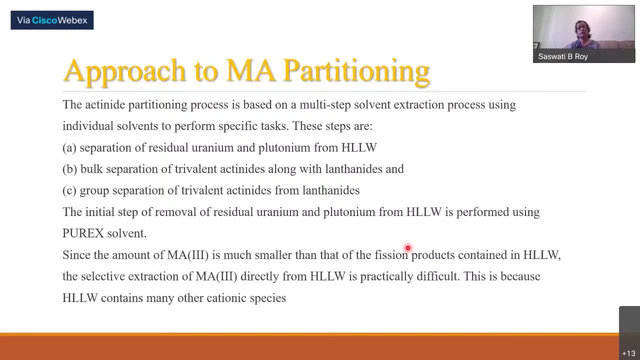 be a group. separation of trivalent actinides from lanthanides. The initial step, which is uranium and plutonium separation, will be by using the purist solvent, means PVP the same way, And since the amount of minor actinides is much smaller, so it will be first taken. 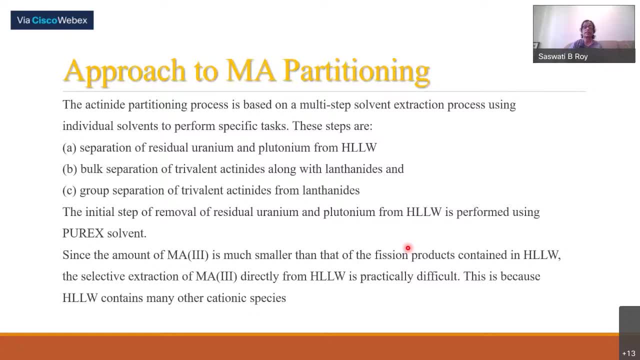 out with together minor actinides and lanthanides, But lanthanide separation afterwards from the minor actinides. it is very much needed because lanthanides are neutronators. So if actinides need to be used in first reactors, definitely lanthanides need to be separated. 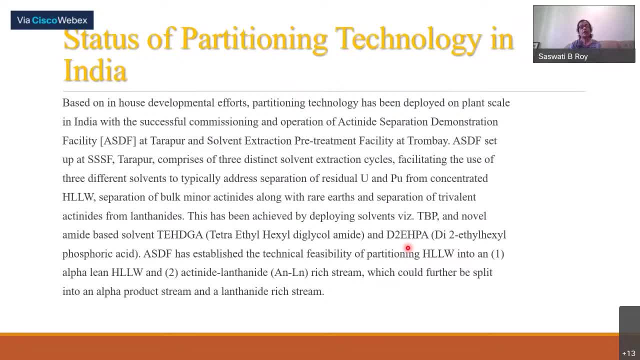 So what is the process? Based on the in-house developmental efforts, the partitioning technology has been deployed on plant scale in India, And there we have seen this in three-stage partitioning. distinct solvent Partitioning systems have been used for partitioning First, the separation of uranium-plutonium. 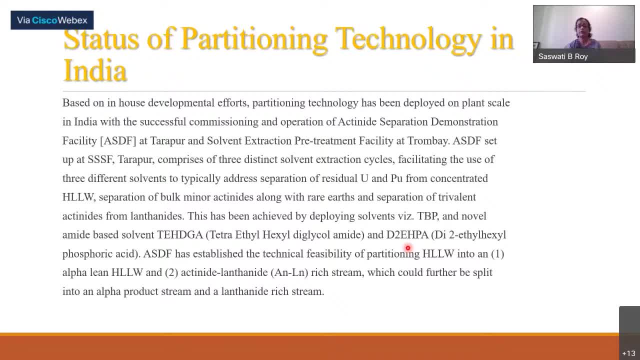 by PVP and then afterwards trivalent actinides and lanthanides. they are separated by TEDGA as a bulk: trivalent actinides and lanthanides. it has been taken out- And then D2EHPA, the DEFY. 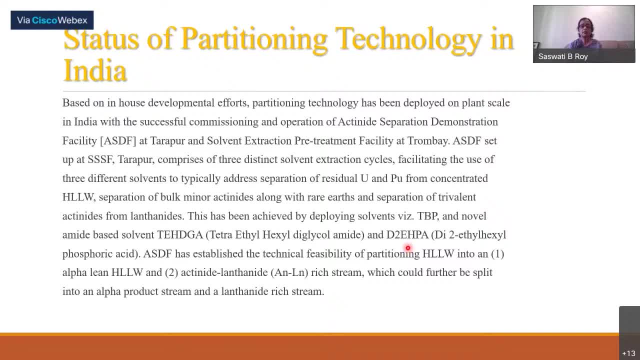 using diethylhexylphosphoric acid. It is used for separation of lanthanides and actinides, So we can get the streams: one stream, high-level active waste without actinides and lanthanides, and then there is one stream where only actinides are there and another stream where only lanthanides. 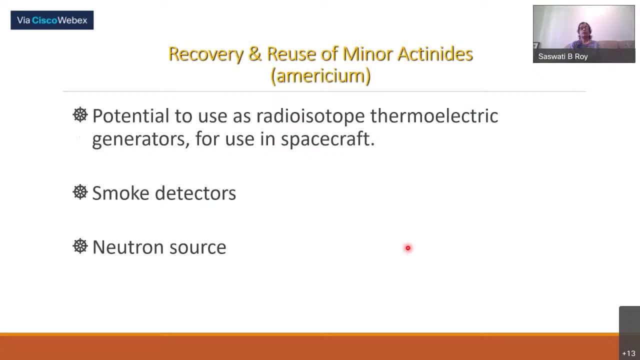 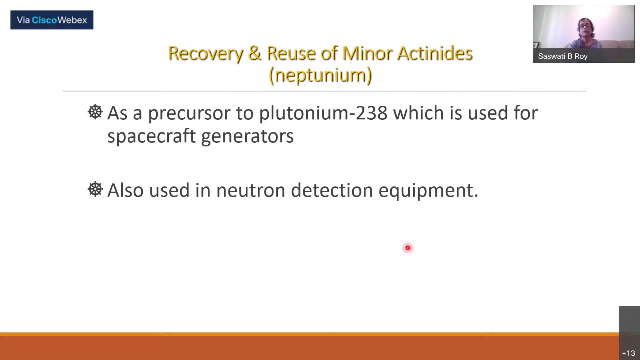 So this actinides, minor actinides, used. you know that americium, there are so many uses, more detectors is a good use of it, And leptinium is a precursor of plutonium-238, also used in neutron detection equipment. So in the summary, if we see this, 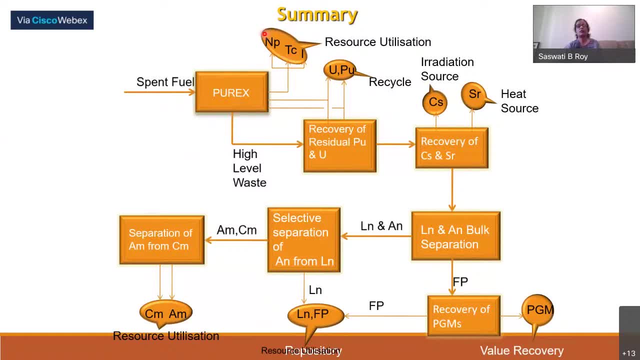 paint field was taken in the puric where we have taken out all our renewable material that we have seen in high levels liquid waste. Now it has been treated with again recovery of residual plutonium-uranium. After removing that, it has been taken for recovery of cesium and strontium. 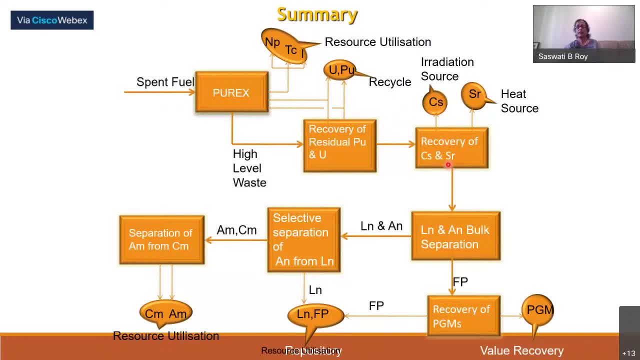 That has been taken out. After that, lanthanide and actinides bulk separation has been done And this bulk has been taken out and that has been separated in the two, two streams: One side your actinides, another is your lanthanides. 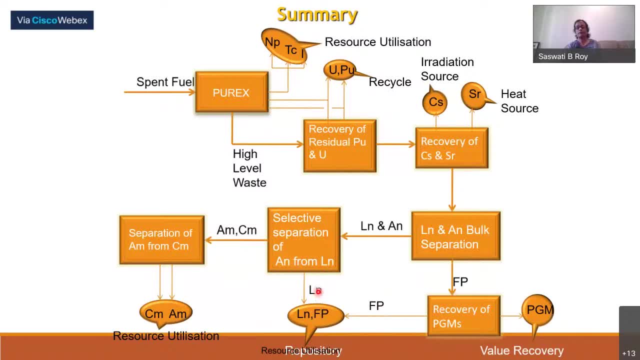 And from there it has been taken for recovery of cesium and strontium, And from the other ends you are getting fission products. Now we have lanthanides and fission products which we have to dispose by conditioning for the repository. So here we can use, as we said, that one conditioning method is. 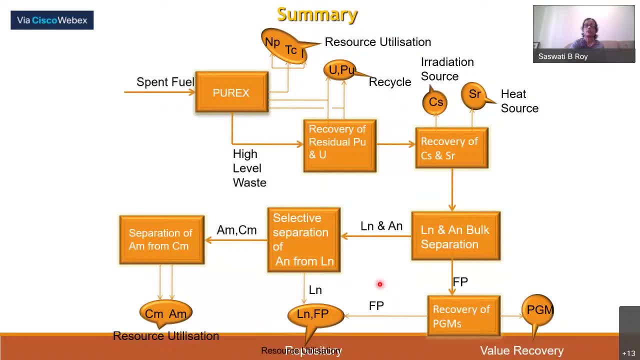 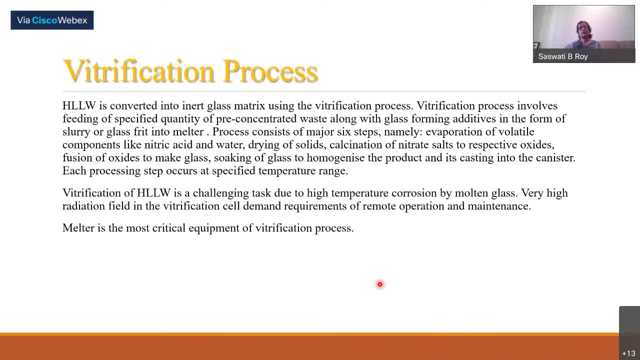 vitrification. So we will see the vitrification procedures: that high-level liquid waste is converted into inert glass matrix using this vitrification process. In this process, the specified quantity of pre-concentrated waste, along with the glass-forming additives like SiO2, B2, or 3, they will be taken and 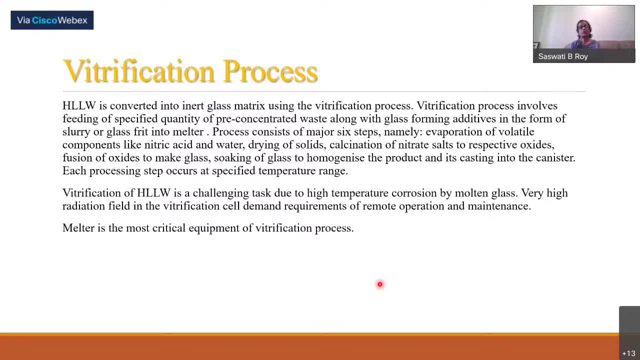 will be heated in a melter. The process consists of six major steps. First is the evaporation, then drying and calcination to nitrate salts, from nitrate salts to the oxides, then fusion of oxides to make glass, then soaking of the glass for homogenization of their product, and then it is casted into the 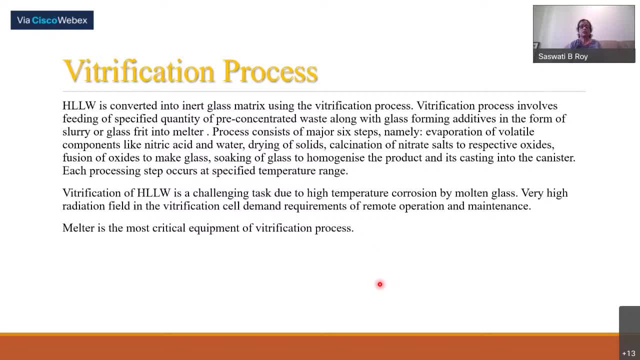 canisters. So here this is a very challenging process, based on the requirement of usage in the high temperature and the corrosivity of the molten glass. So here this is a very challenging process based on the requirement of usage in the high temperature and the corrosivity of the molten glass. 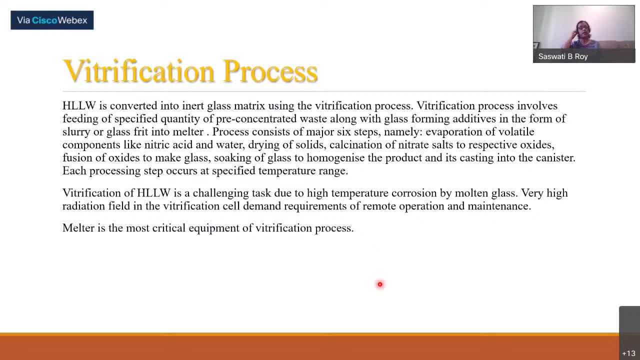 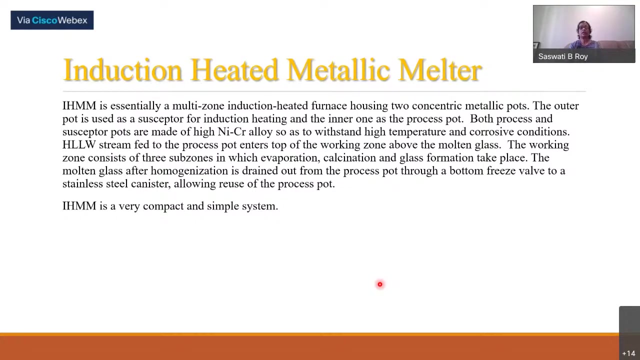 you need totally remote maintenance and operation and melter has to see all these abuses. so melter is the most critical equipment here. so depending on the melter design, there are two, three different types which we are using. one is that induction heated metallic melter. This is the most simple one. Here there are two process pots. One outside is a scepter. 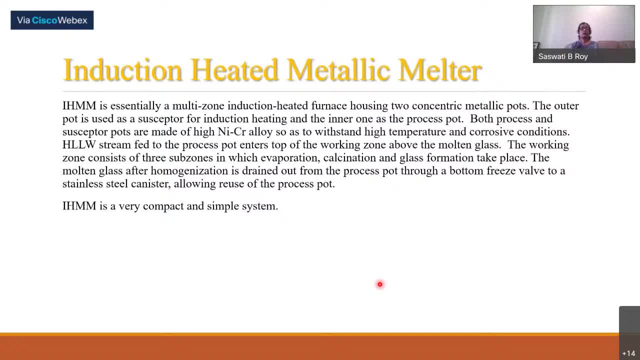 and the inner one is the process pot. This scepter and process pot, both are made in high chromium alloy because they have to withstand high temperature and the corrosion resistance. In this we can see the temperature of the different processes like this: Initially, when we do the evaporation, that may be around 150.. From there drying is around 250. Then 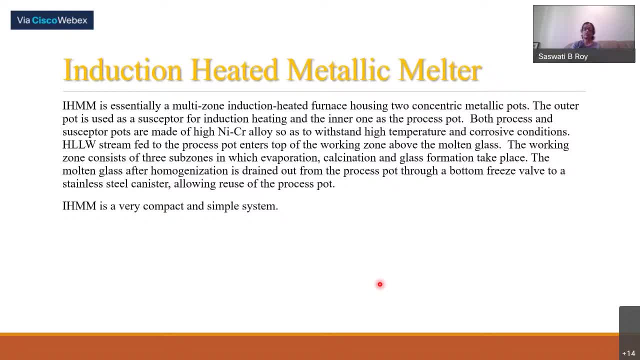 from drying to next stages, including fusion. that will be around 800.. Calcination will be up to 800 and then fusion will be in the range of 900. And after fusion, homogenization of the process. homogenization is in the range of another 25-50 degree centigrade. So you can see it's. 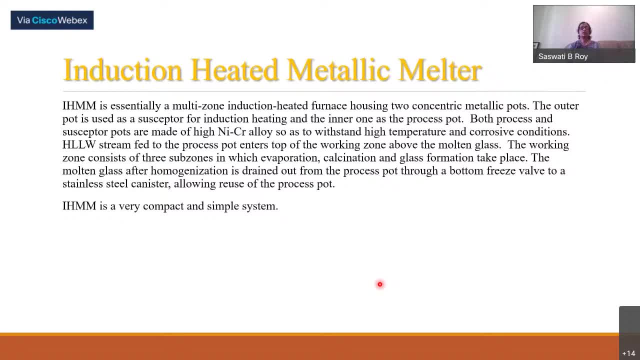 a huge temperature. To see this, we need a specific grade of material, So nickel, chromium alloy is being used. And then, after completion of the process, like all this, first it will be taken glass-free, it will be taken inside the process pot and we'll be feeding our 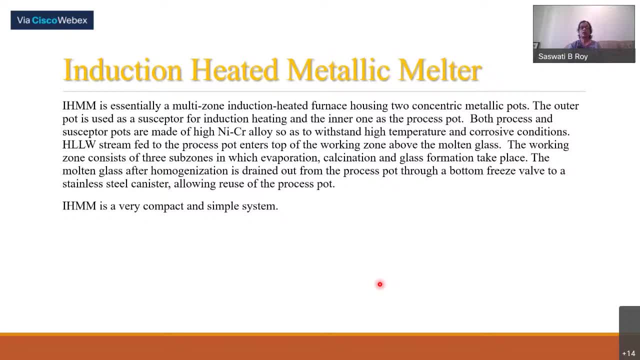 concentrated high-level liquid waste And with temperature. we go on processing different steps And at the end, after homogenization of the glass, this will be taken out from the process pot to a bottom freezer valve to the stainless steel canister allowing. 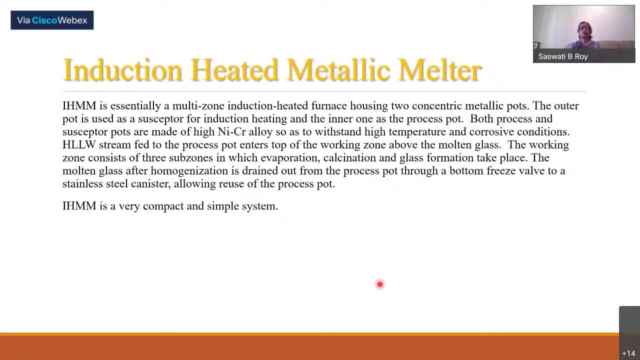 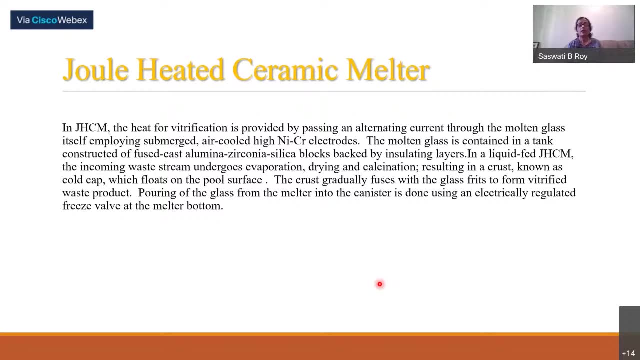 reuse of the process pot. Now, this process was very simple but, as you understand, because of this corrosion and high temperature, it's very difficult to process the glass. So we are also carried out a process of refitting in a way that we do it from outside. So we take all the storage, everything we get. 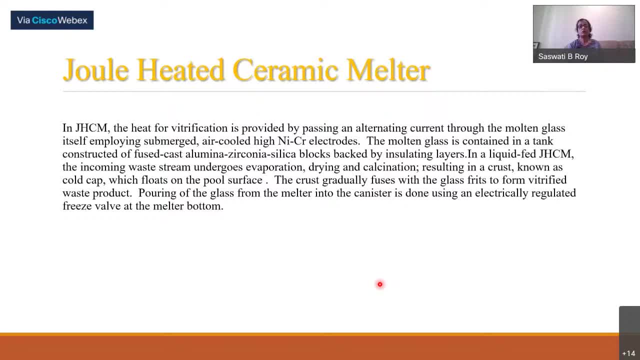 as the temperature. This metallic melter changing is a requirement. So they went for the ceramic melters. Here the heating is by the joule-heated. so this resistance and using nickel, chromium, alumina, zirconia, silica blocks backed by insulating layer, Here also in the 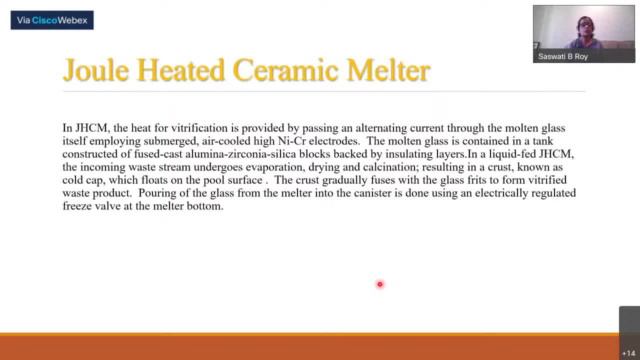 similar way the frit will be made and after that it will be taken down. after the frit going through the all the six steps, the frit, once it is homogenized, whole glassy material, it will be taken out in that through the melted bottom. 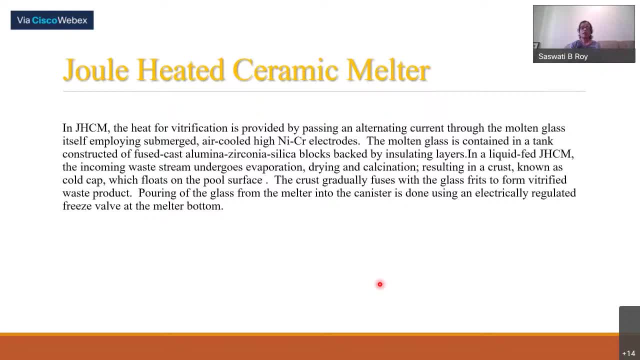 using electrically regulated freeze valves. Here actually, the, as you see it is a ceramic melter, so a process pot corrosion is reduced, but this electrode life in this high temperature, in this corrosive atmosphere, again as a limited point, and also during decommissioning, because of this very bulky nature of the. 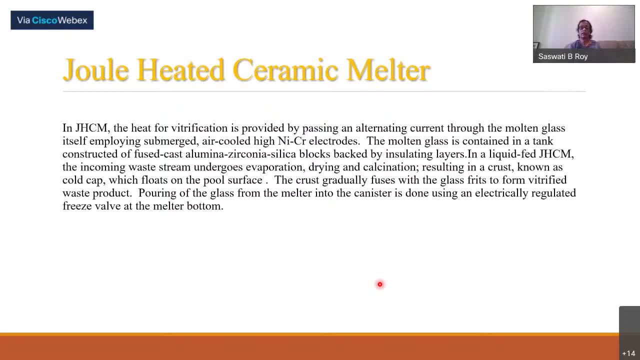 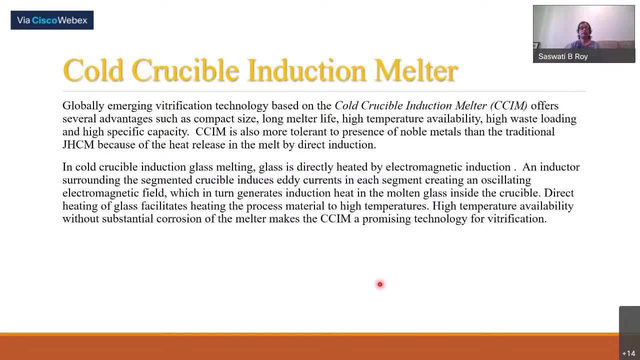 ceramic ones. It shows little difficulty. so some more developments have been done, and the recent one is the old crucible induction melter, when the crucible is metallic but due to specific arrangements, like what we used to do in our uranium melting- not melting uranium production- the reactor is made of mild steel but it 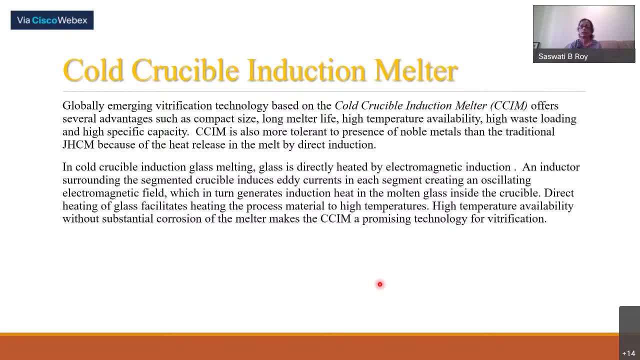 is lined with refractory material during the process, so that we said here also: during the process. the cooling arrangement has been made in such a way that your pot- metallic pot- is protected by a thin layer of cold glass and inside that glass there is the molten, main fluid material. 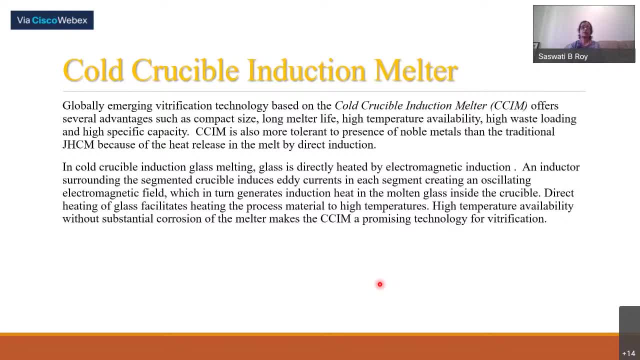 which is at high temperature. so this is this. temperature attainment is again by induction melting, and so the crucible is cold and inside high temperature directly you are getting by induction melting, so it is good to maintain the higher temperatures and this is suitable for this. platinum group materials for. 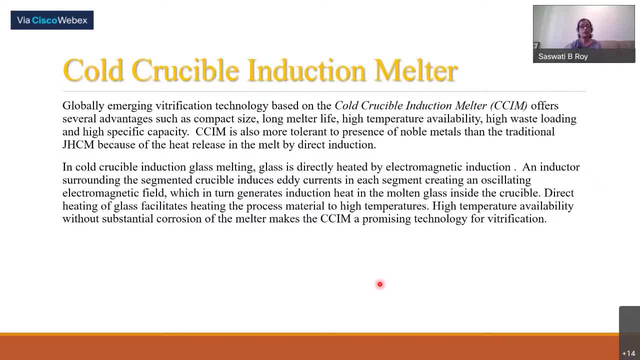 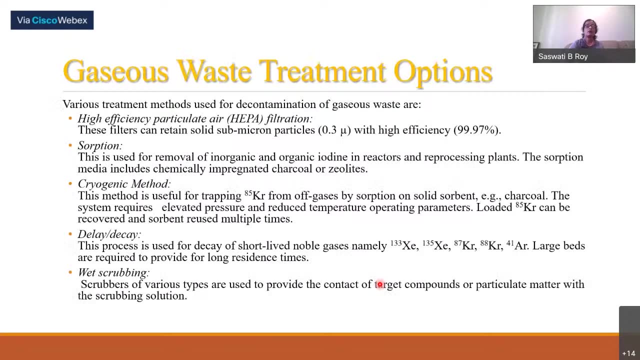 this high temperature attainability- so high temperature availability without substantial corrosion of the melter- makes the CCIMA promising technology for the electrification. so this is our the latest one. during this process and many other processes we generate a lot of gaseous waste also which needs treatment. the various treatment methods used for this: decontamination of the 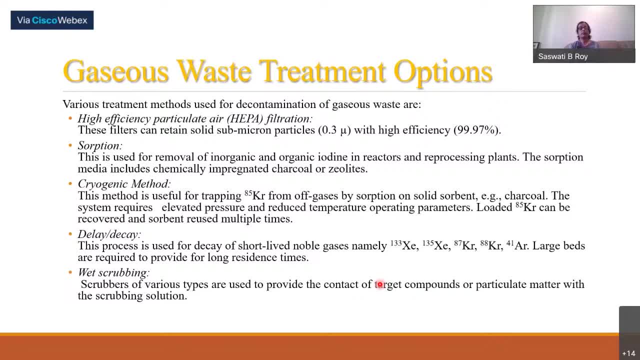 gaseous waste that high frequency particulate air filtration. this filter is a HEPA filter which can do a sub micron particles with high efficiency sorption. thus this is used for the removal of inorganic and organic iodine in the reactors. the sorption media includes: 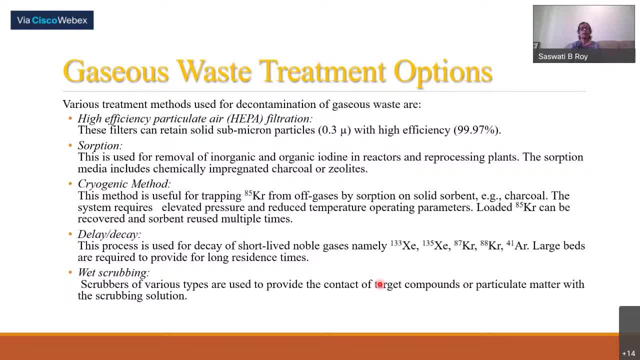 chemically impregnated charcoal or GLA. cryogenic methods. this methods is used for krypton, where we need elevated pressure and reduce temperature, and this this is also again in the solvent, like charcoal, and this can be dissolved for reuse of the krypton. and it can go on. 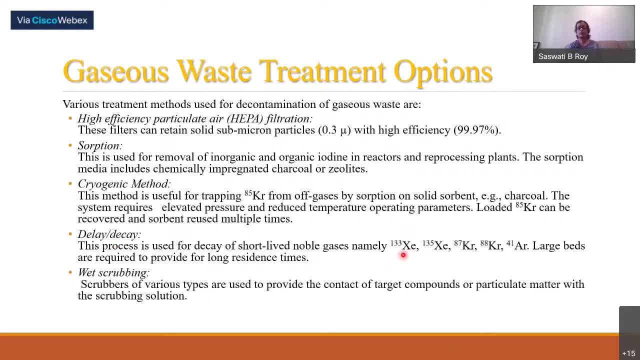 delay and decay is another methods, which is for gaseous products like xenon, krypton, where large beds are provided to which, as the person, they get delayed and decayed, and weight scrubber is a universally used process for many processes or radioactivity, including our conventional chemical gases. 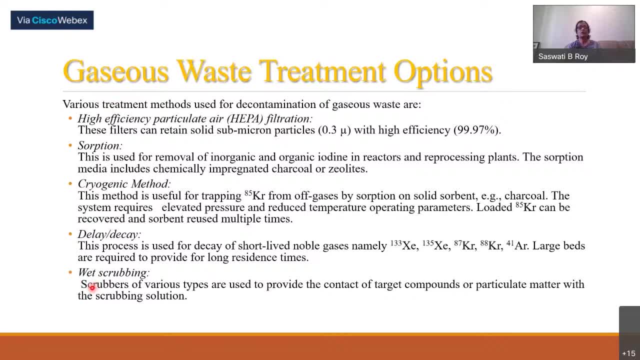 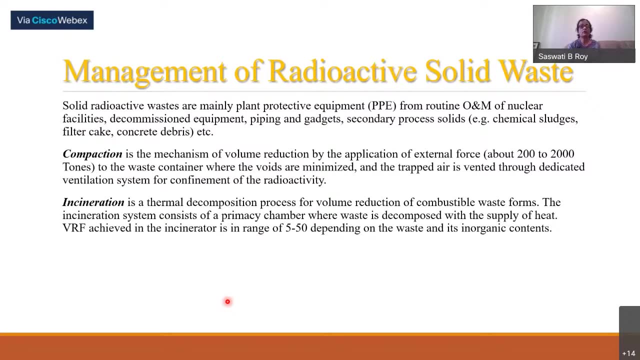 also so these are few methods which are being used for this, depending on the requirements, as it is a fit, suitable. and next is your management of the radioactive solid waste. this project is taking place from the, from the system, which is primarily plant protected equipment or routine maintenance items. maybe for the decommissioning equipment, piping gadgets like this, or secondary process solids like air filter, cake, concrete debris, etc. so there are a few methods or the basic tool which you do is compaction. so reduce the volume and it also allows to reduce the volume and 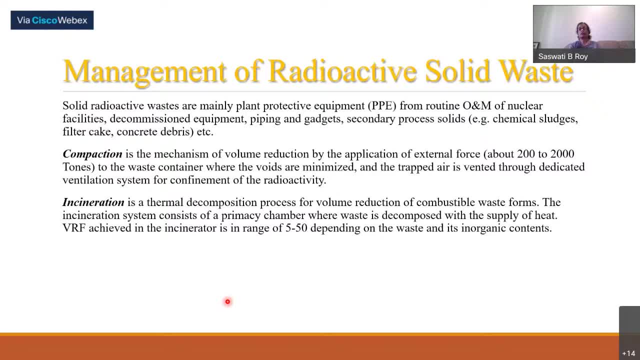 it also allows to reduce the volume and incineration, and now it is mostly plasma incinerators used so that you can go high temperature without emitting any toxic gases. so there also you get a good amount of volume reduction and if there are contaminations, this can go for. 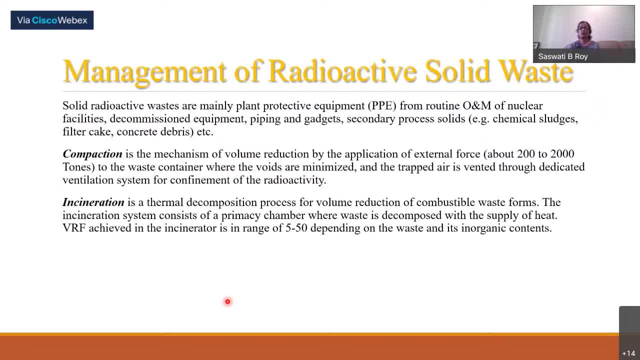 acidization type of things where you can remove this contamination, or a separate additional blasting methods where you can remove your required loose contaminations inside the enclosed atmosphere. so there's a very few processes which we use and in incineration actually liquid also can be incinerated, like your organic liquids that also can be incinerated, depending. 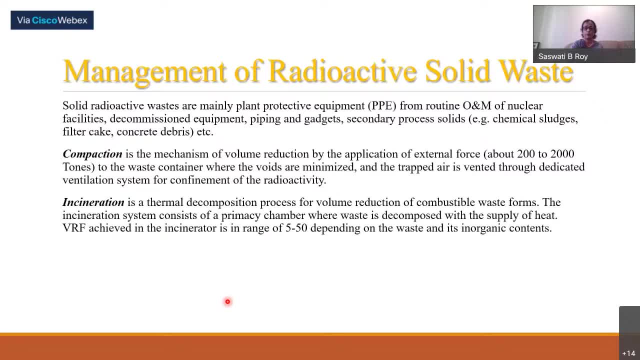 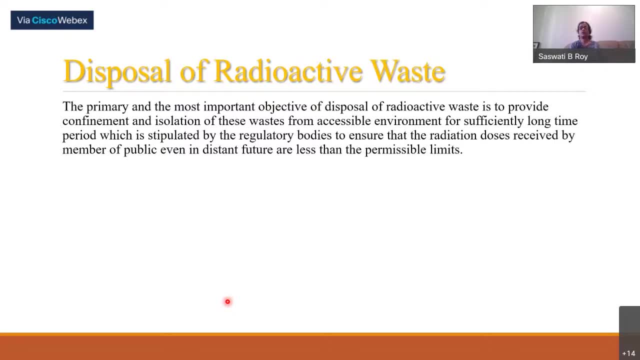 on the specially designed condition you once they have been now made in the solid forms, compacted forms from the liquid, from the gaseous or from the solid itself, after compacting and decumptioning. now this has to be disposed. so the primary and the most 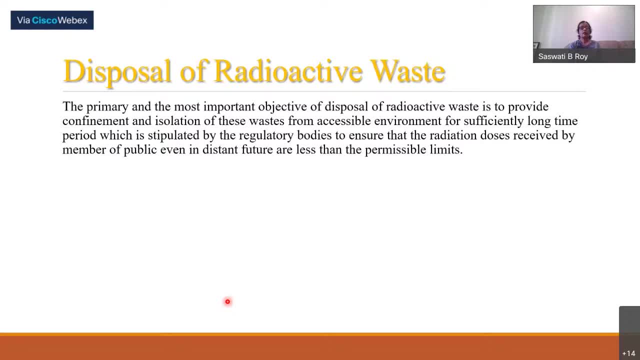 important objective of the disposal of radioactive waste is to confine and isolate this waste from the accessible environment for sufficient period of time, which is stipulated by the regulatory bodies, to ensure the use of radioactive waste in the environment and to ensure that the waste is not released to the public. and to the public and to the public. 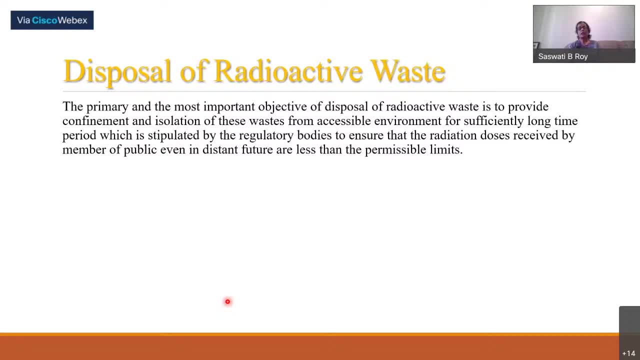 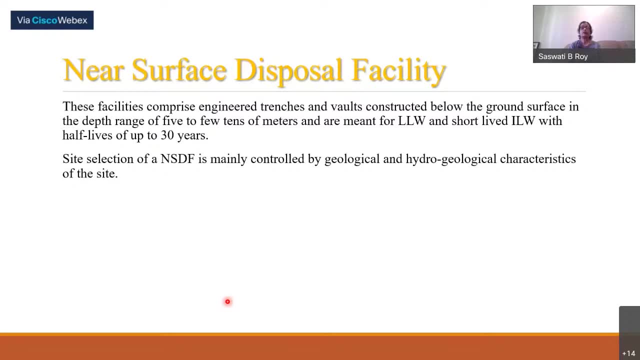 so that the radiation does not reach to the member of the public even in the distant future, and this is less than the permissible limit. so, considering this requirements, there are few disposal facilities are being used. the one which is for the, as we said, low level or the intermediate level is 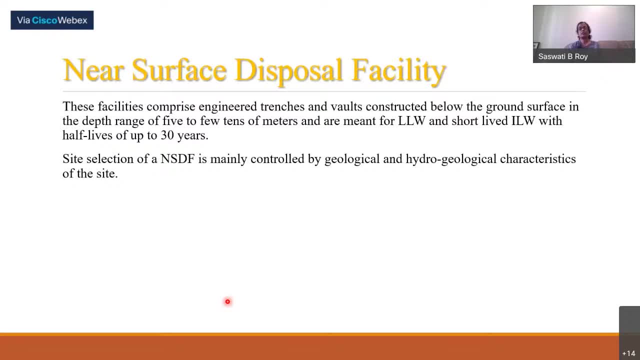 near surface disposal facility. this facility is used for the use of the air, but it is a is generally used for electromagnetism or geotaphic speakeasy ability as well, and one of the of the most important facilities said by the, by the, the. 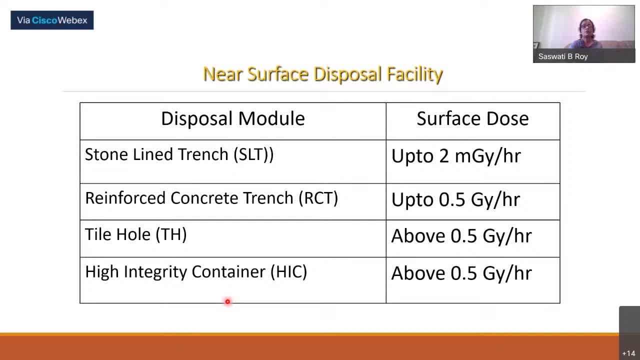 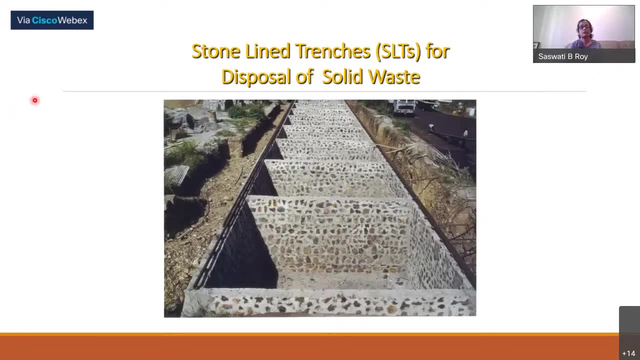 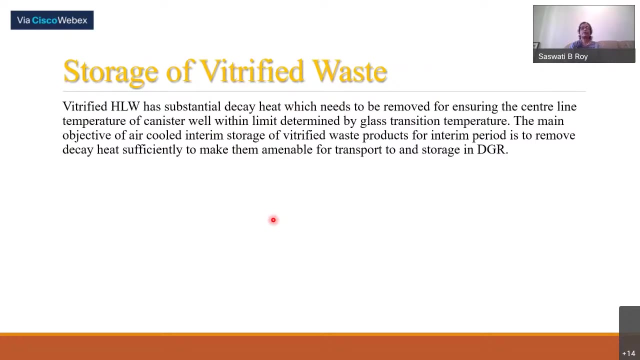 comment: didn't like stone-lined trenches, reinforced concrete trenches, dry holes, high-intensity containers, depending on the surface contamination. So this is one of the trench which is just made for filling your solid waste And vitrified waste, as we said. 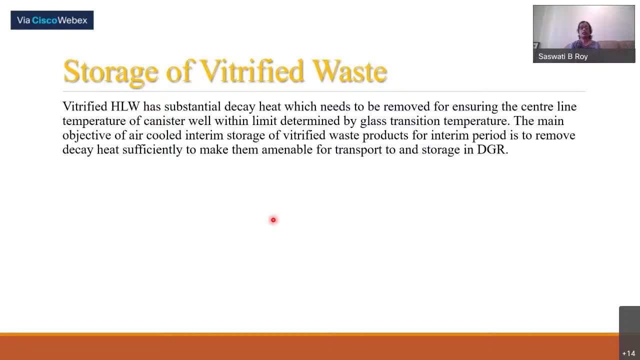 that is in the solid in the canister. but what is needed- heat removal- is a requirement. So for this heat removal we have to keep it in a storage, intermediate storage place where air-cooling arrangements are provided. So these are specially designed. 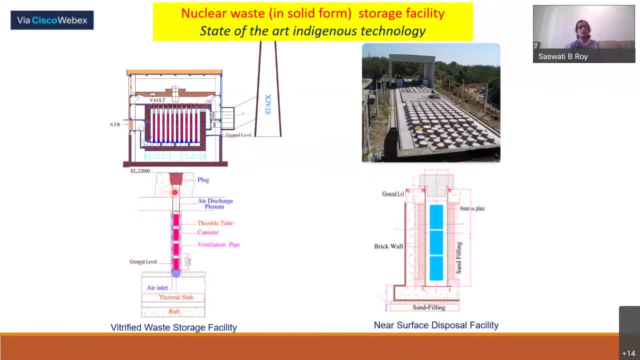 You can see where this. this is just above the ground. This is not. this. one was below the ground for the near surface disposal facility, where we have made holes and then your drums have been kept. These holes are lined with stainless steel. 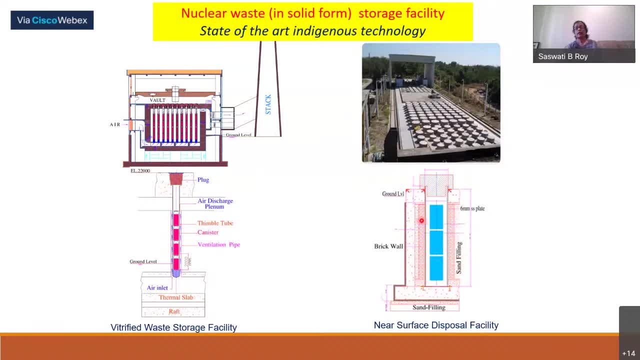 Then you can see, here on the other side, you have your brick lining, Then you have your sand filling, So this may be around five meters depth, And at the top we have concrete planks. So, as and when required, we can even take them out. 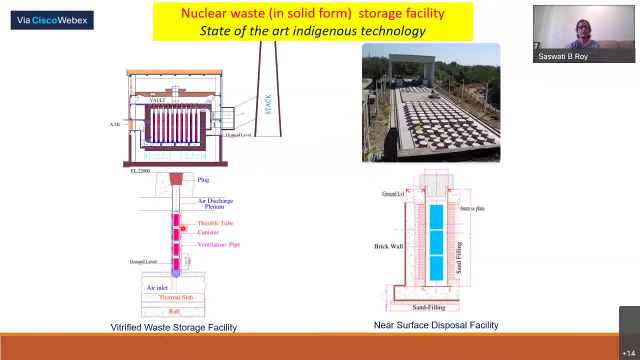 And, in case of this special vitrified waste storage facility, these are just above the ground where we can put similar, you know, drums, lining will be there And air is being passed through these areas, which will be passing through all these drums. 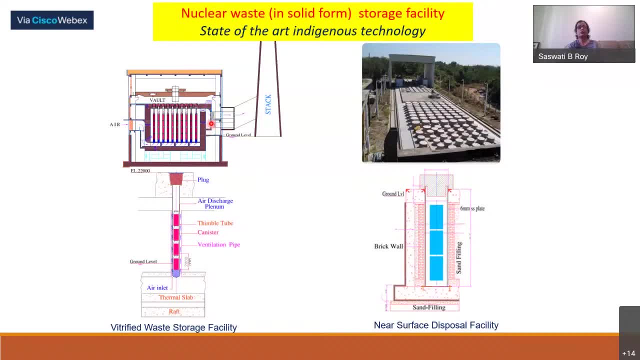 and cooling them. And this air, with proper regulatory arrangements, will be exhausted through stacks. So this cooling arrangement is a requirement for keeping the chemical stability of the material inside so that temperature does not increase beyond the restricted. so that temperature does not increase beyond the restricted point. 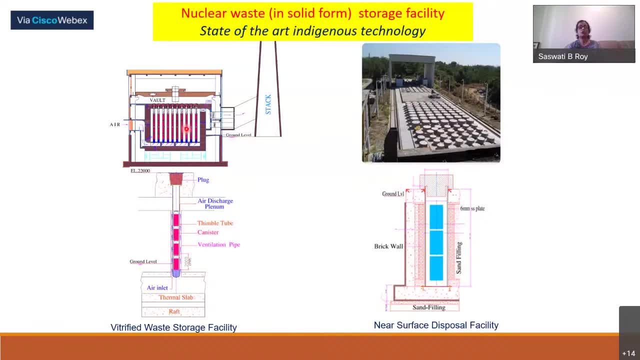 And these arrangements- you know special arrangements, so we will try to reduce the amount of the material or the time need to be kept here. So that is the reason why we are doing individual and the bulk separation of nucleides from high-level waste. 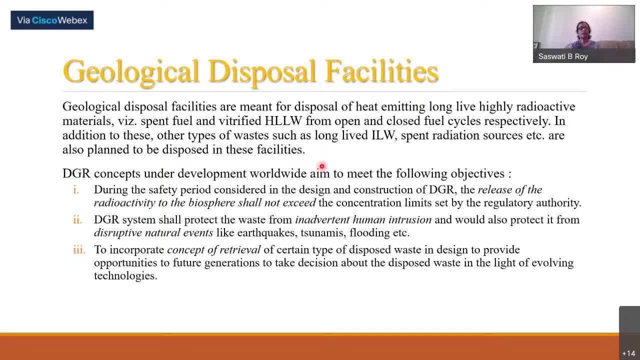 And the final depository is the geological disposal facility And the final depository is the geological disposal facility. So that's the concept for this geological disposal facilities. So that's the concept for this geological disposal facilities that, during the safety period, considered in the design. 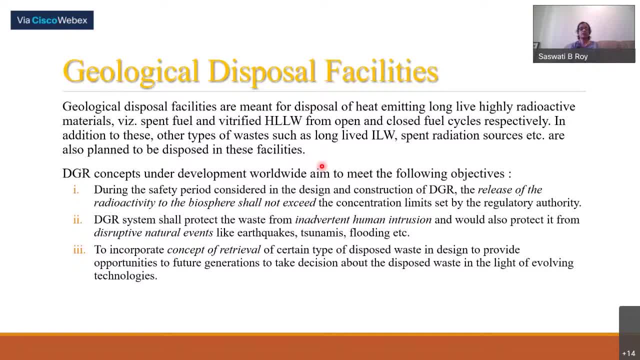 and construction of DGR. the release of the radioactivity to the biosphere shall not exceed the concentration limits set by the W2B authority, And DGR system shall protect the waste from inadvertent human institution and also protect human life, And also protect human life. 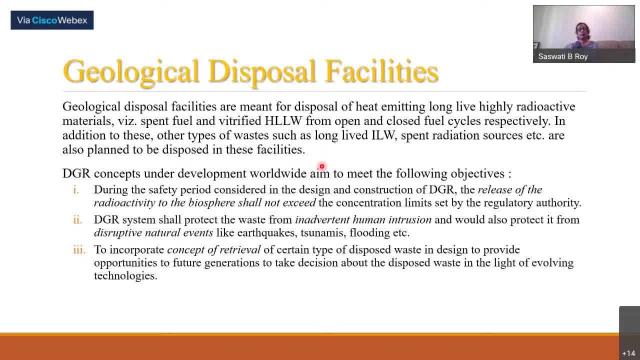 And also protect human life, to protect from the disruptive natural events like earthquake, tsunami, flooding, and also to incorporate concept of retrieval in future generation, if they wanted to reuse it for something else, for something else or to do it some other treatments. 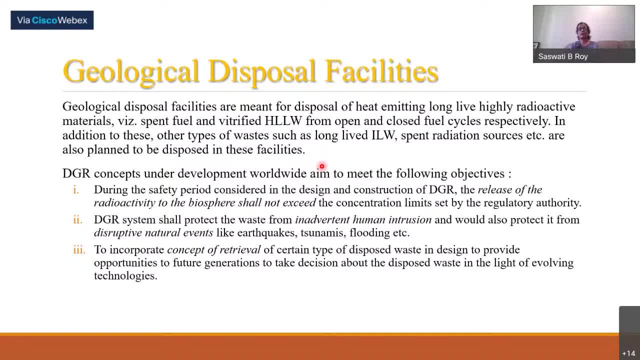 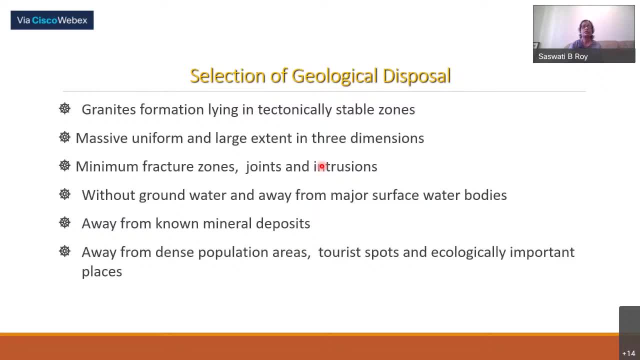 that facility also should be there. So, based on all these things, this is being designed And there are few considerations, And there are few considerations for the site, as we all know that it has to be away from the known mineral deposits are from dense population, away from major surface water bodies- minimum. 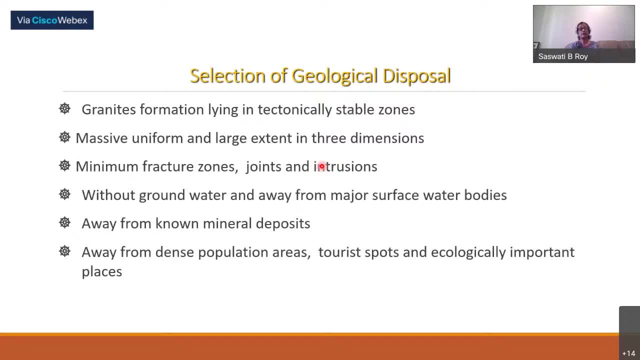 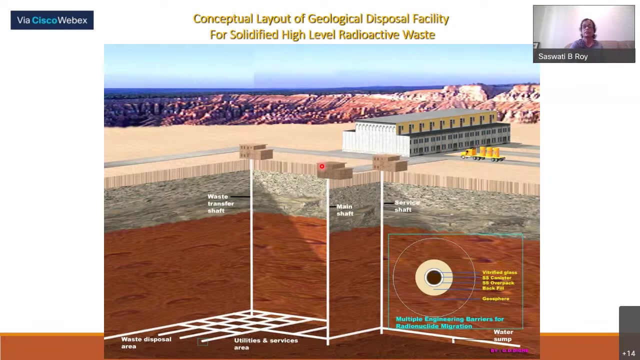 fracture Jones: massive, uniform, large extent in three dimensions and granite formation length in technically stable zones. it has to be a very stable zone, so this is for the final disposal. so with that we conclude today. these are all views of the artistic views, how to put them inside the zoological deposit worlds, and this is your multi-barriered. 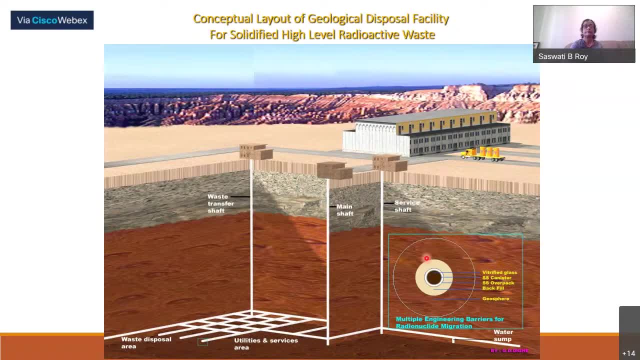 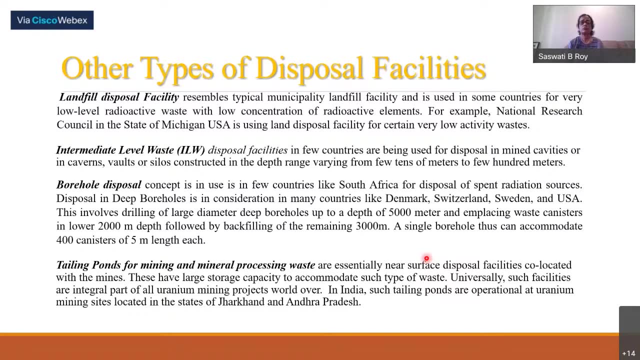 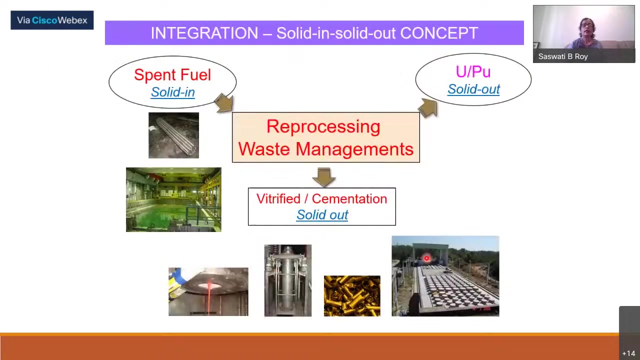 canisters, other type of this world facilities which are much lesser, the active materials like land filling, intermediate level waste filling, bore will disposal or tailing ponds, which you have already discussed. giving our other points at the end there is a recent train, but it has to be integrated, but solid, solid. 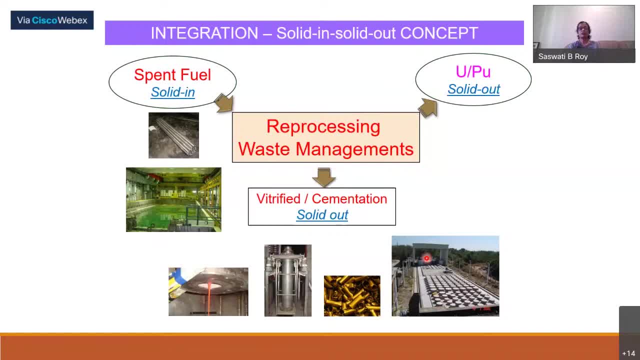 in solid out concept where the processing and waste management should be integrated, where the solid as a waste or the spent- well, we will come and this rectified- are cemented. college will go out after management like this: near surface or other canisters are for your which, if I, storage facilities. so 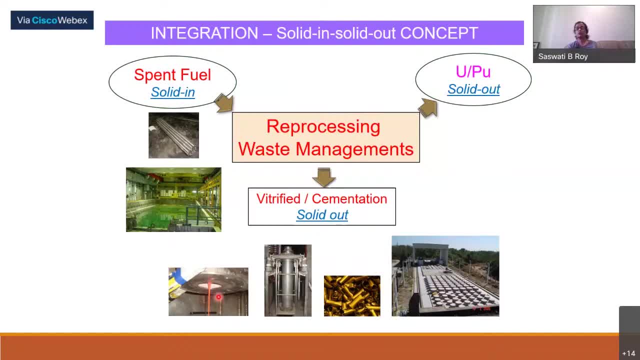 integrated plants and nowadays, more requirements. this is a neutral thank you. with that I end, and before I close this, I just want to thank you very much for your attention. Thank you, I just wanted to have two important points to tell you. First is that I told you I will give you some reference books. 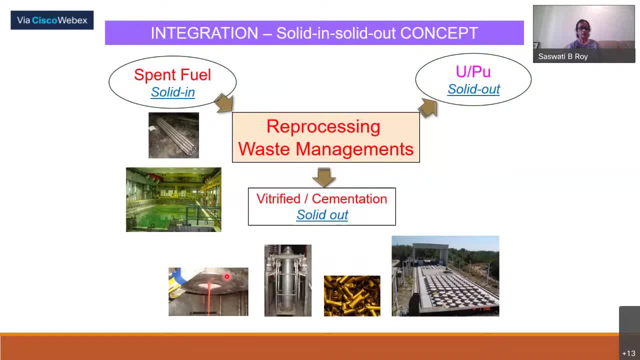 So the reference books which I have consulted, the first one is the Nuclear Fuel Cycle, the book going to be published by HB&I, which is under publication stage- You will not get now but maybe shortly you will get it- And various bulletins of the IONCAS. 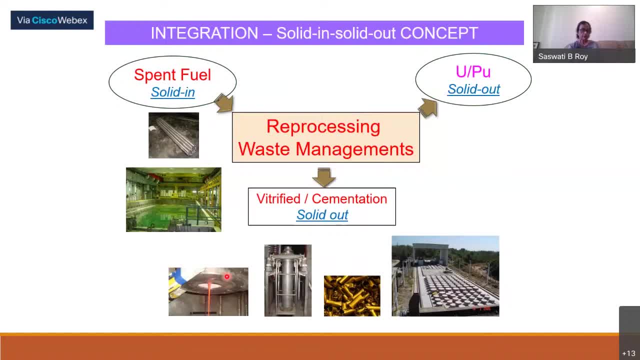 specifically the bulletins of the Nuclear Fuel Cycle, Industrial India, Atomic Energy Supplements for our old documentation. Then Nuclear Chemical Engineering- Benedict and Pickford, Uranium Overprocessing by Clegg and Foley, Uranium Production Technology by Harrington And really Secondary Resource Processing. 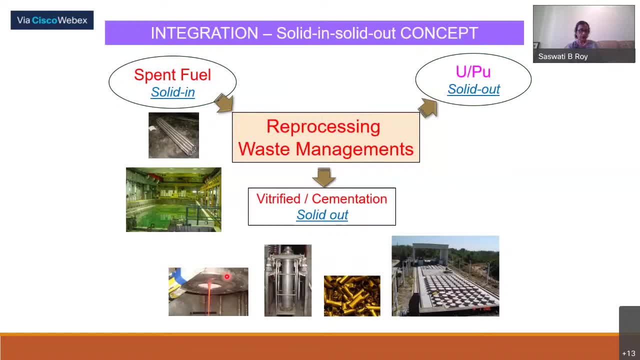 by Sikhi Gupta, Ed Singh, Neutronium Metallurgy in India by Pierre Roy and Ganguly. Uranium, the book by TK Smurthy. And I was telling I will give you some general references also, but this is quite a long list. 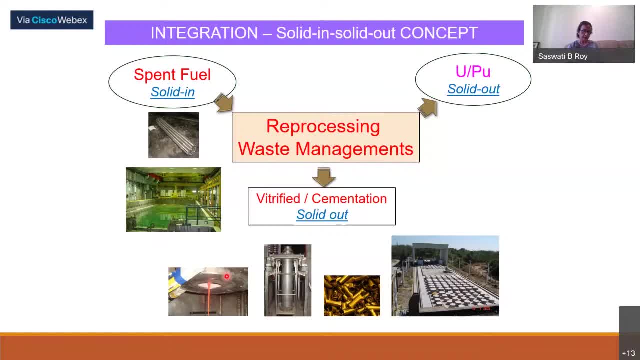 You can see this Journal of Nuclear Materials. there We have published Our Various Papers on Morphology and the Thorium Activity. So with that, this reference point, we end and I go to the Acknowledgement parts. Here I first acknowledge: 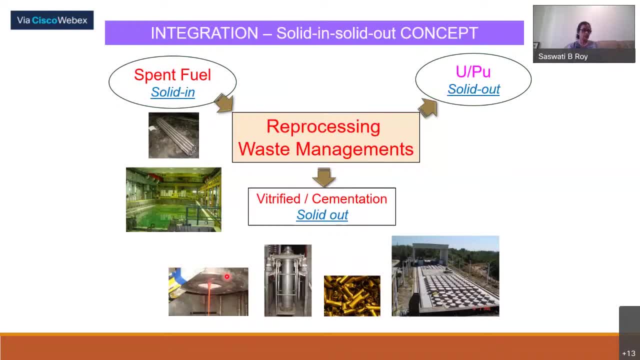 Sri SN and Sri TK Smurthy. They are the former directors Chemical Engineering Group. Today they are no more there with us, but they did Many earlier jobs and they have kept all this information For us, you know, and the 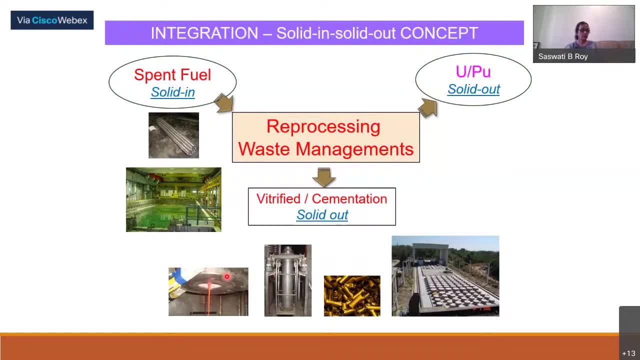 I acknowledge the help received in making my slides And the presentations following names: Uh. Sri Amitabha Roy, former CENRV, and his colleagues. A DVD. Sri ML Sahu and his colleagues. Head MIND Dr Srinivas. 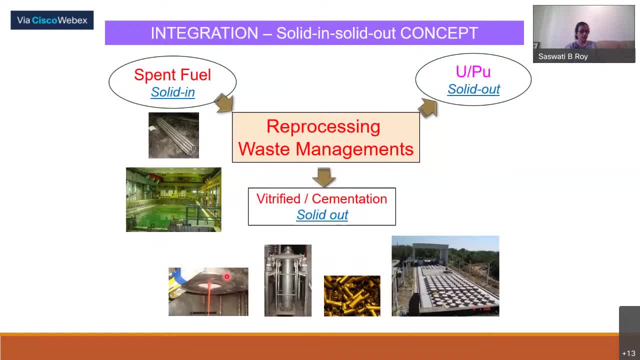 Dr K Rao, Mohammad Sirajuddin, Amit Patel of MIND, Sri Kanwar Raj and his co-workers. Today's all the work is from their work only. Whatever. we have discussed their work and their writer, Sri Kanwar Raj, and all his colleagues, including Sugilal and Smita. 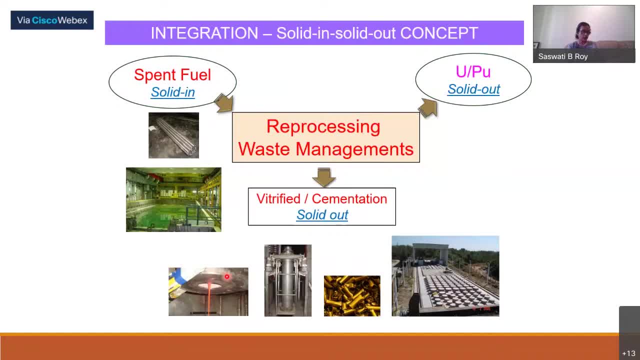 Then I acknowledge Sri Kalburgi AD CTD, Sri Rajesh Kumar Heavy Water Division, Sri Sanyal- now he has retired- Former DC NFC For our information on zirconium We also acknowledge from IGKRC. 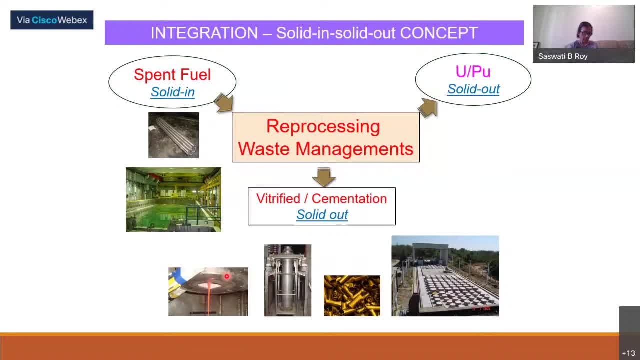 Ramananda Rao and Shiv Raman. At the end, I must thank Professor Kumar and my son Aroni Roy. Without them, nothing would have been possible, And if I have missed any names, that is only due to my failure. 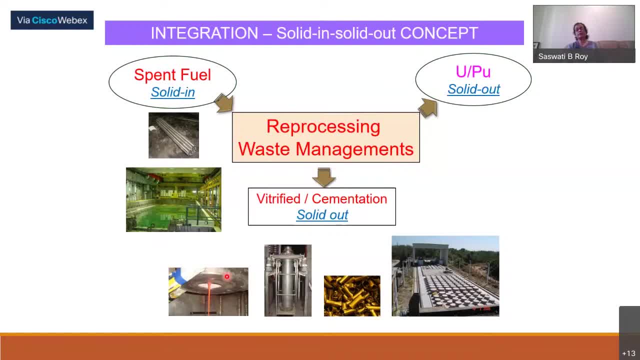 It is not an intentional, Please forgive me. Thank you Over to Professor Kumar. Thank you, Professor Roy, For describing the journey of Uranium, thorium and other actinides From cradle To grave. Cradle is the mines and graves the repositories. 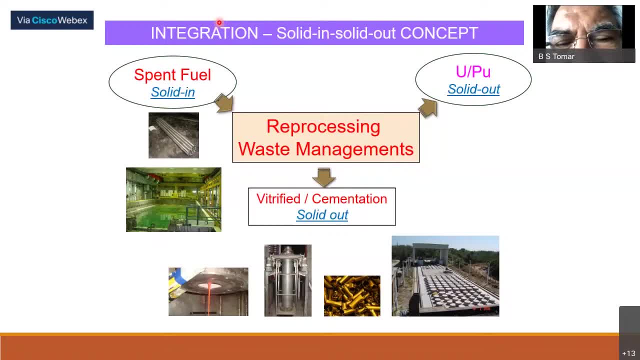 And in the process we Harness the nuclear energy by using them Without leading to any Radioactivity in the environment. So now we go for any questions. If the participants have any questions, You can write in your chat box So that you can. 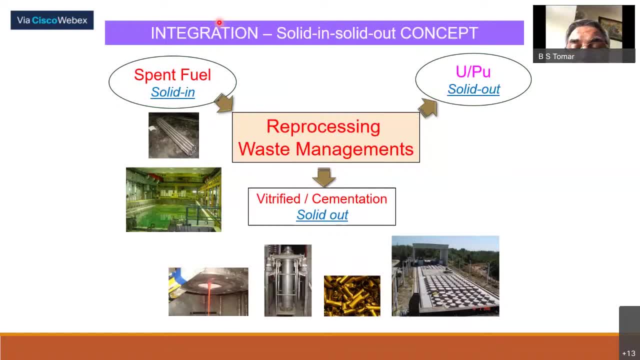 Try to answer them. If you have any questions, please write in the chat box. Yeah, there is a question. Can we get the study material for nuclear fuel cycle One to seven? Yes, you will get it, The book which is going to get published by HBNI. 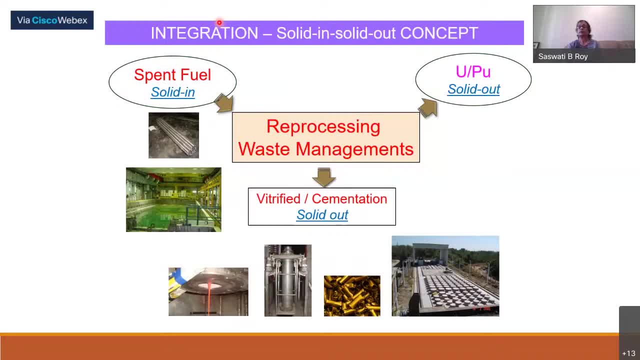 Okay, So that may take some time, Maybe a few months time. Yeah, With the slides, the slides. So whatever you have made After sanitization, if it can be, because there are a few things which may be correct. 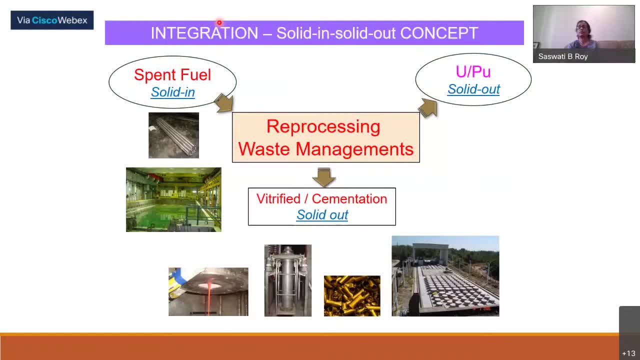 Correct. So I have to just check it up. And then that is what I was telling. Yeah, If in a day or two, if you could send them, then I could, we will post on the site. I, I will. I will just check it up from that point of view. 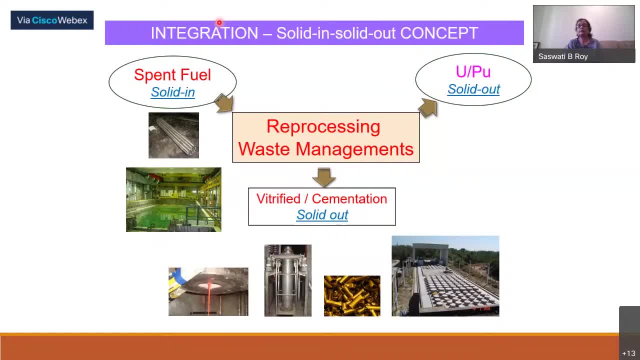 If it is physical, I'll definitely share No issue, Sure, Sure. Okay, there is one question: are the deep geological repositories currently in operation worldwide? No, not that way. Operationally You cannot see. Yeah, I think none of the DGA are operational but Finland, Sweden. they are in a very advanced 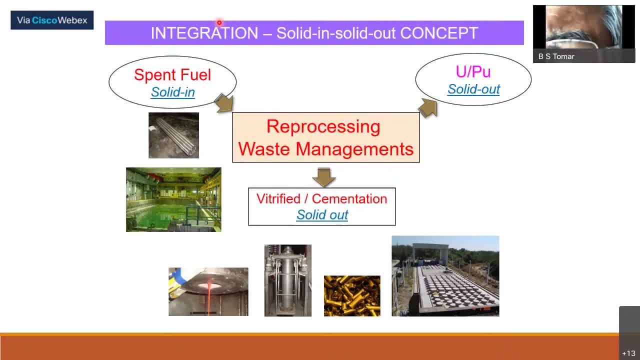 stage of operationalizing their repositories, So maybe in a couple of years time. the fastest to go is Finland. finland, they have already made an advanced repository. any other question? so, if there are no further questions, i would like to thank professor shashwati rai for giving a detailed description of the 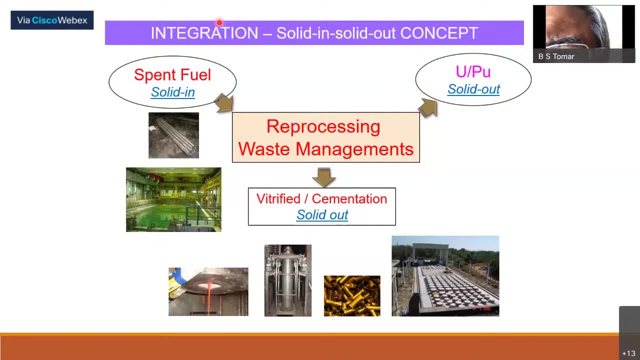 nuclear fuel cycle from mining, milling, fuel fabrication, fuel reprocessing, waste management and finally, deposition in the repositories and also getting lot of valuable materials from the high level waste in terms of the useful radioisotopes. so thank you, professor rai, for your lectures and i would like to- yeah, i would like to. 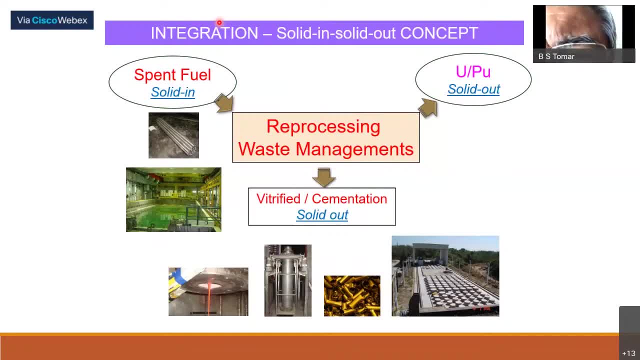 tell the participants again. repeat that adding a feedback form has been sent to you by our central office. kindly fill that form and give it to us. send by email to me so that we can know how. how was the course taken and what were the difficulties. we can try to solve them in the 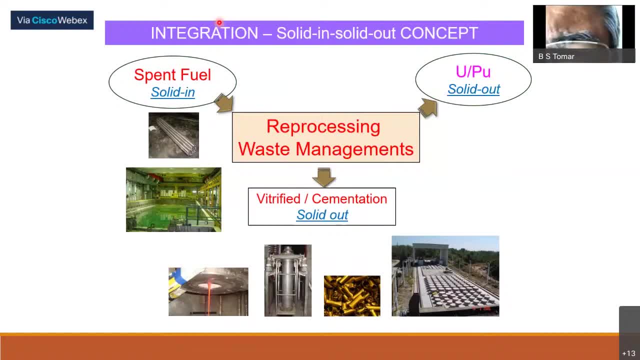 subsequent lectures, subsequent online courses and secondly, those of you who would like to submit the assignments, please do the same by 31st of may, because after that it may be difficult to accept the assignments. you have one week's time to submit the assignments you want to earn the credits, and we will have a viva voci on 4th of. 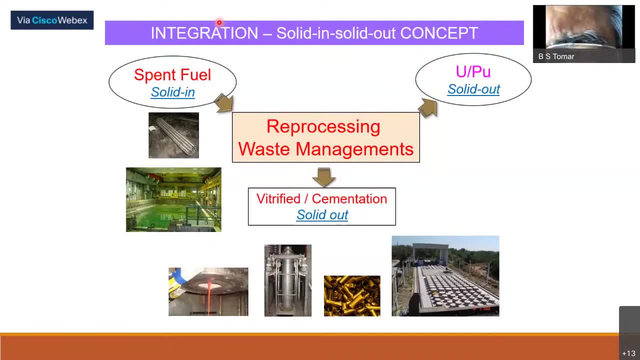 june and when, in the validity function on 11th of june, the participation certificates will be given away in virtual mode. they will be posted to you later on. so wish you all the very best and i hope you enjoyed the the course. you do send your feedback how it can. 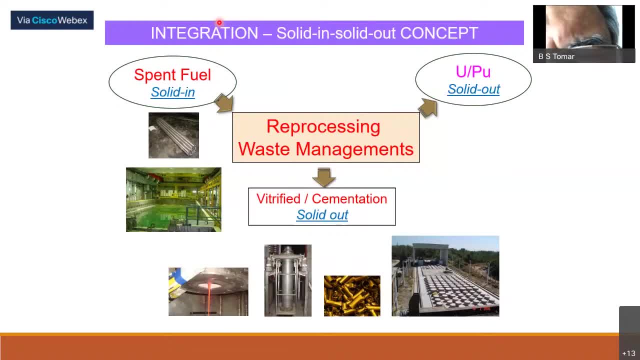 we can improve upon it. thank you and all the participants, participants, and it was nice. yes, yeah, many of the participants very active in asking questions and, yeah, yeah, yes, i wish them all the best and let us keep our contact. if anything is needed, we will be. yeah, you can write to us, to me, about any other aspect of the program.